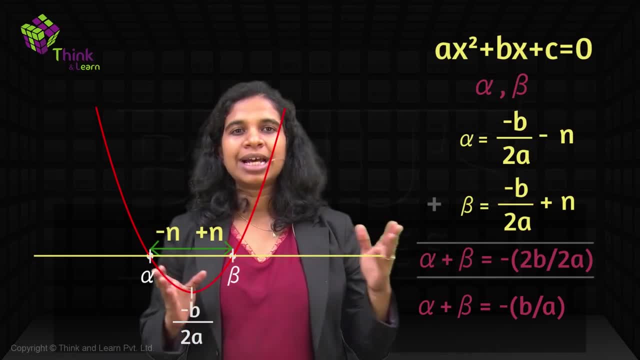 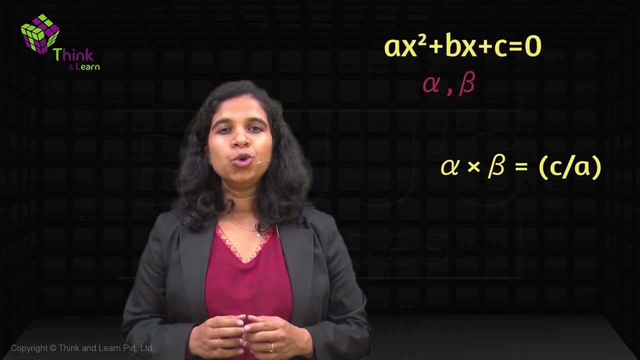 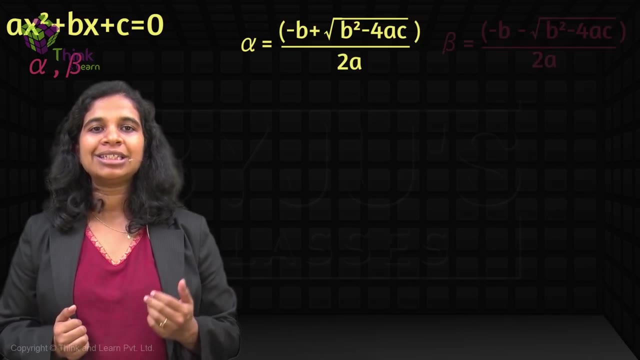 2a, which is minus b. So alpha plus beta is minus b by a. Alpha into beta is equal to c by a. Again, if you use your quadratic formula, take alpha as minus b plus root of b, squared minus 4ac by 2a, and beta is minus b. 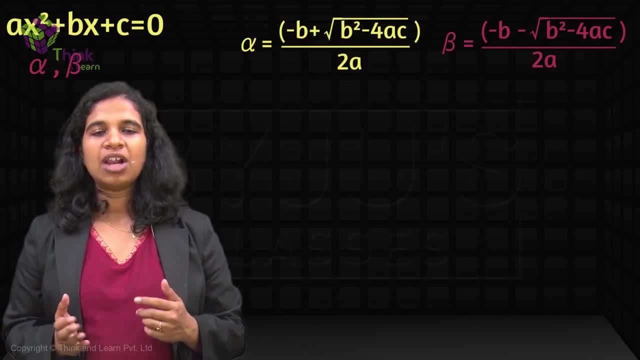 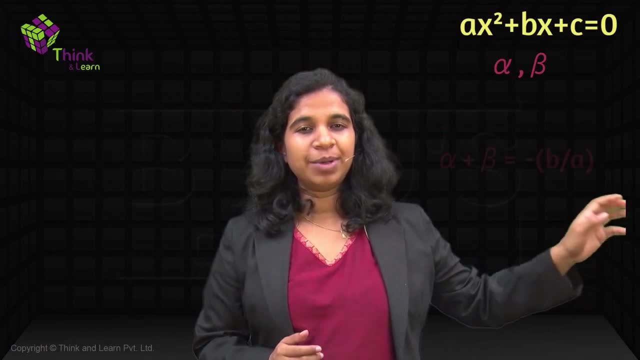 minus root of b. squared minus 4ac by 2a, You will get: alpha into beta is equal to c by a. You can see the calculation here. So those are the two equations that we have: Alpha plus beta is minus b by a and alpha into beta. 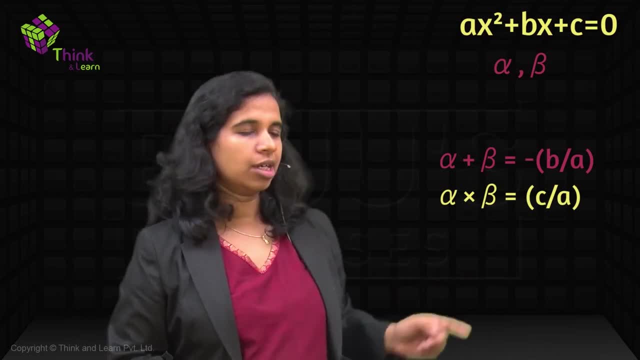 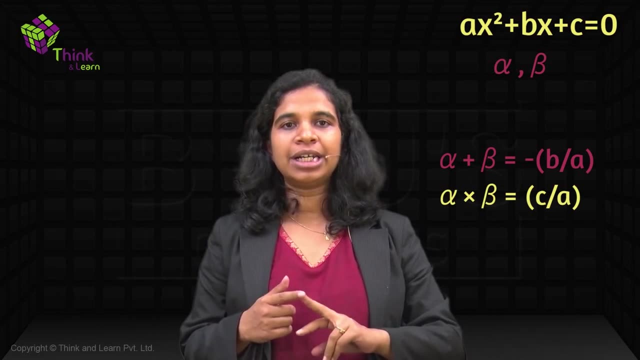 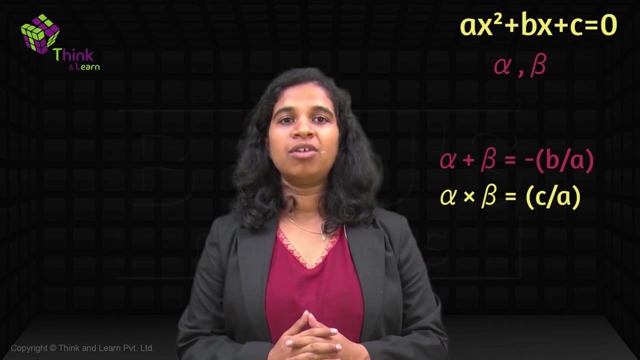 So we have two equations here and two variables. a, b and c are known to us because the equation is given. So the two unknowns here are alpha and beta. We have two equations and two unknowns. We know that we can solve them to get the answer. So you will get a value for alpha and a value for. 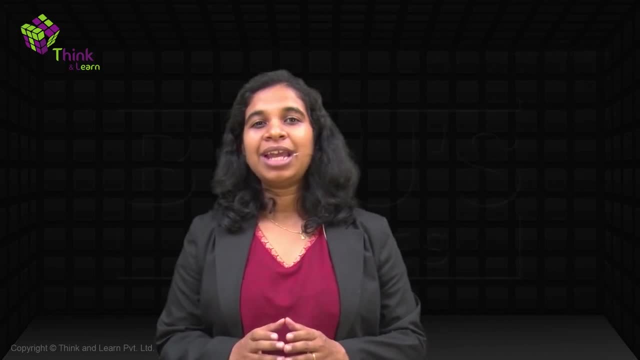 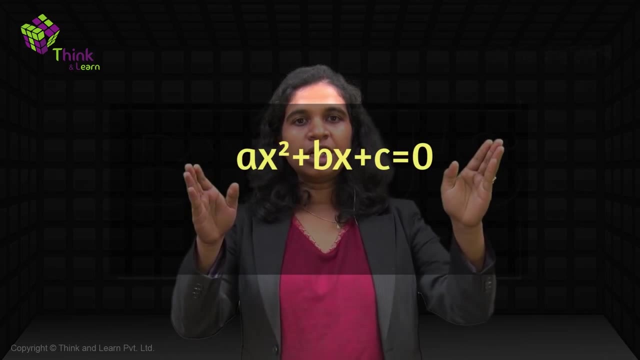 beta. Now, actually, the same logic can be extended to even higher order equation. Just think of what we did. We had a x squared plus b x plus c. The first term was equal to a x squared plus b x plus c. 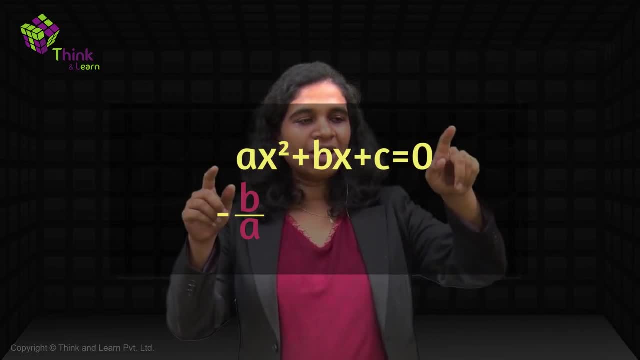 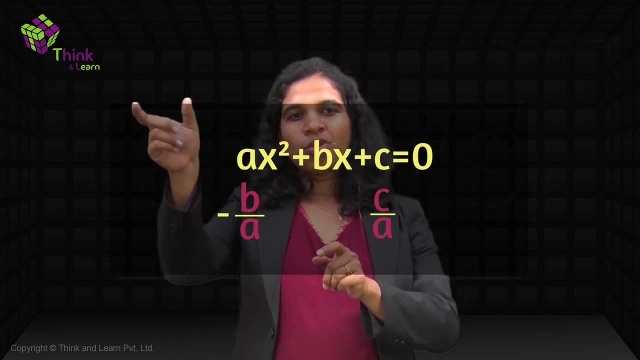 It was nothing but b by a with a minus sign Minus b by a. The second one was c by a with a plus sign, Correct: In the first one this value was equal to alpha plus beta. So when my roots are alpha and 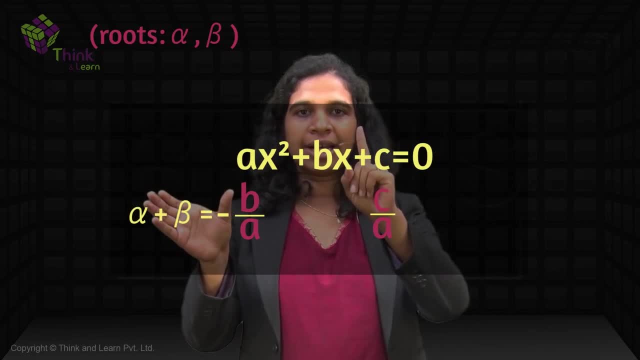 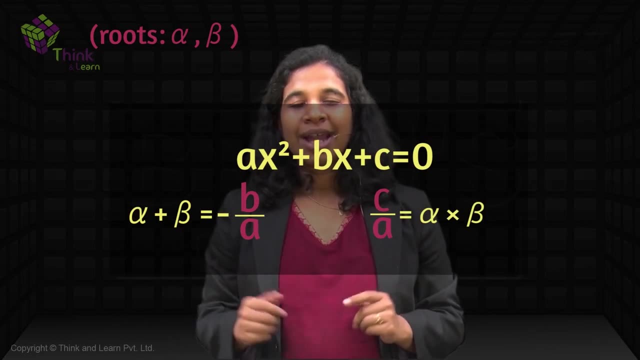 beta. I can say this is sum of the roots taken one at a time. Right, I am taking one root at a time and adding them Now. c by a was nothing but alpha into beta. So I can say this is sum of the roots. 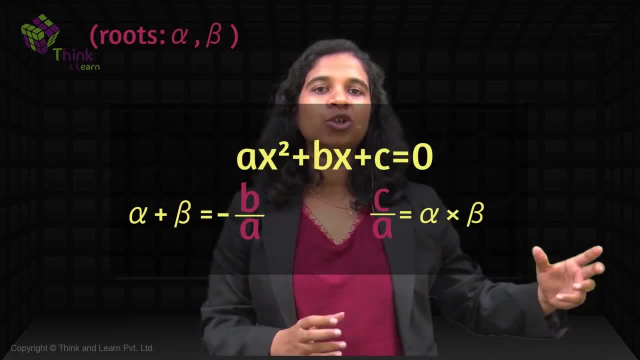 taken two at a time. I am taking two, two roots at a time and adding those pairs Here. there are only two roots, So there is only one pair, So I am adding it once. It will be more clear when we take a. 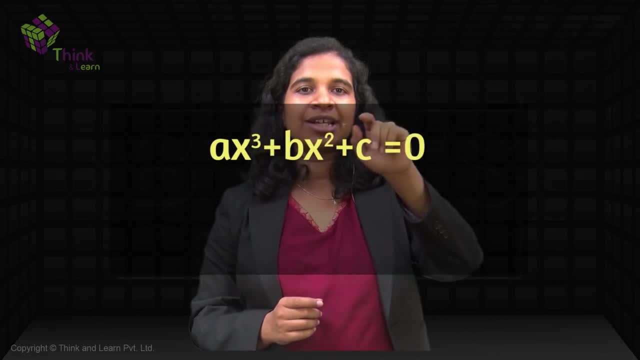 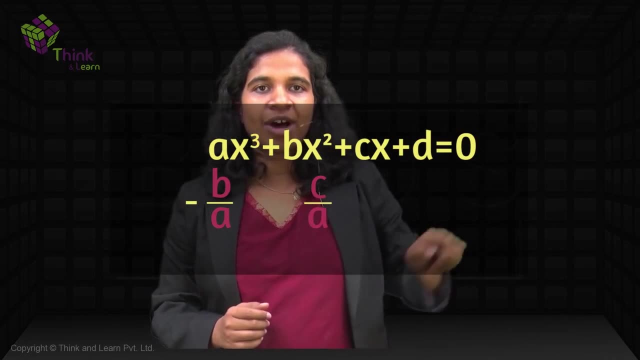 cubic. Let's convert this to a cubic. So I will make this: a x cubed, plus b x squared, plus c x plus d. I am going to add: So minus b by a remains the same, C by a remains the same. Now we will have: 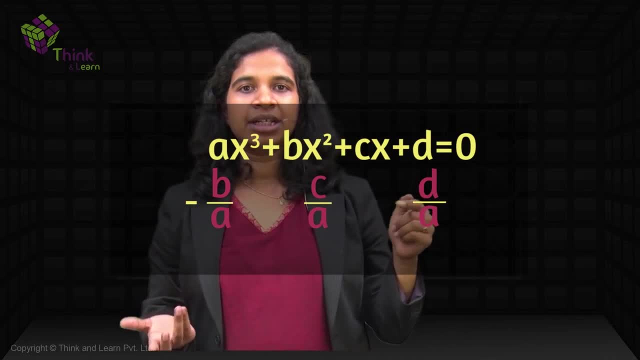 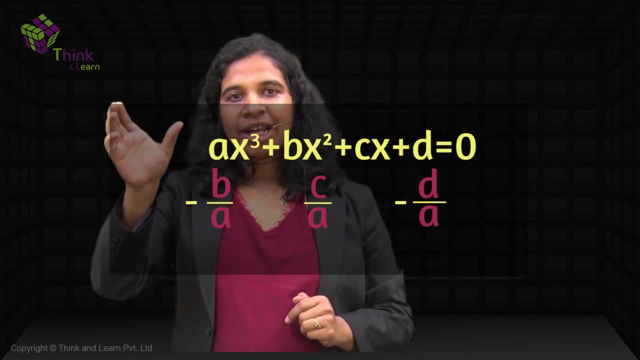 one more thing, d by a, which will have a plus or a minus sign. Minus, right, You can see. it is alternate negative and positive signs. Now, the first thing is sum of roots, taken one at a time. The second thing is taken two at a time. The third thing is taken three at a time. 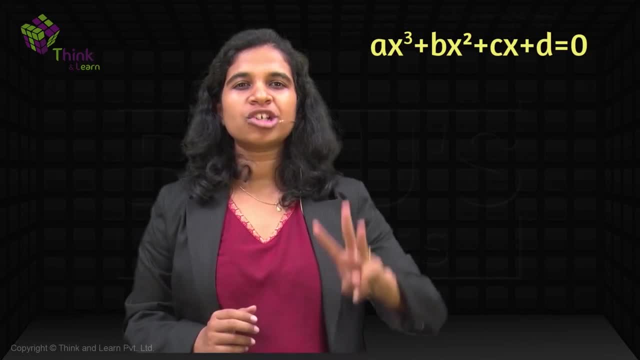 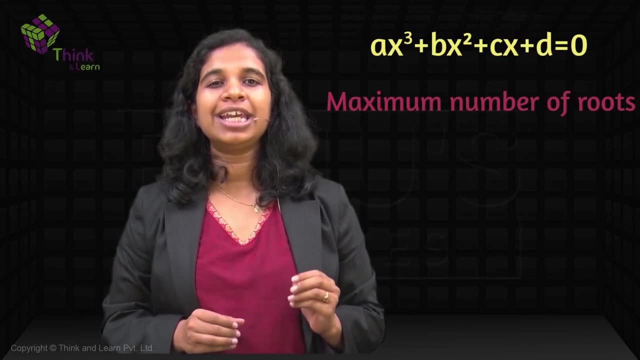 And so on. So now a cubic equation will have three roots. When we do higher order equation, you will see the maximum number of roots that any equation can have will be equal to its degree. It will always be equal to its degree. Sometimes they will be real, Sometimes they will not be. 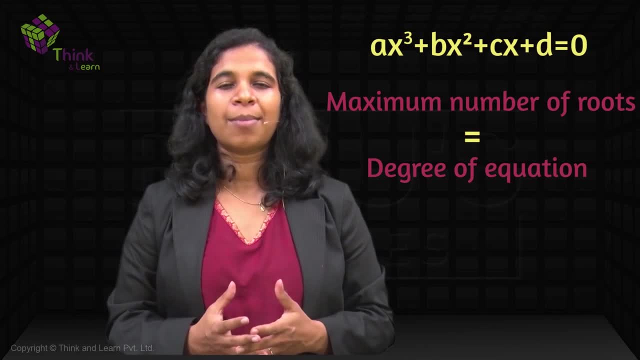 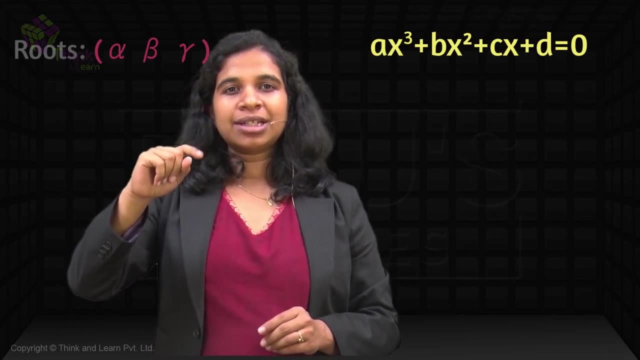 real. So that is why I am saying the maximum number of real roots. Sometimes they might be less than three, It will be equal to three. So let's say alpha, beta and gamma are the three roots. Now the first part is sum of the roots taken one at a time. So I will take them one at 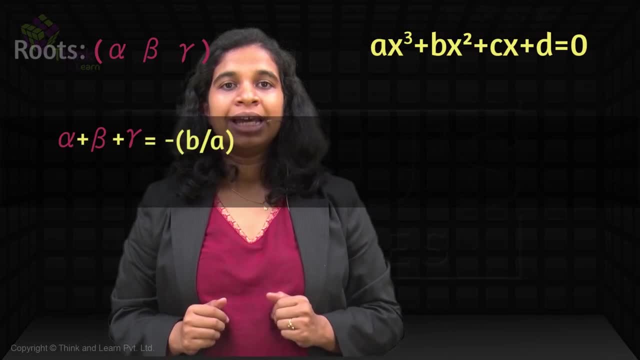 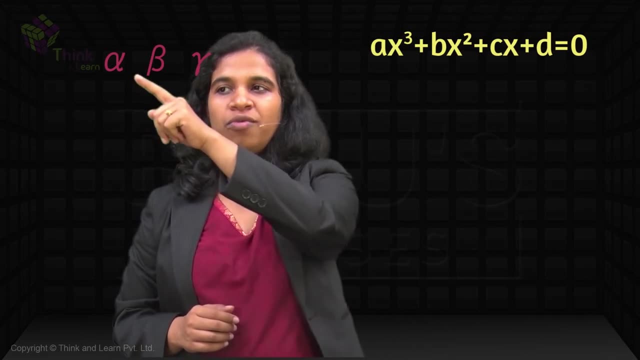 a time, plus beta, plus gamma. Very simple: Equal to minus b by a. Next is sum of roots, taken two at a time. So take groups of two. We have alpha, beta and gamma. How do we form groups of two? We? 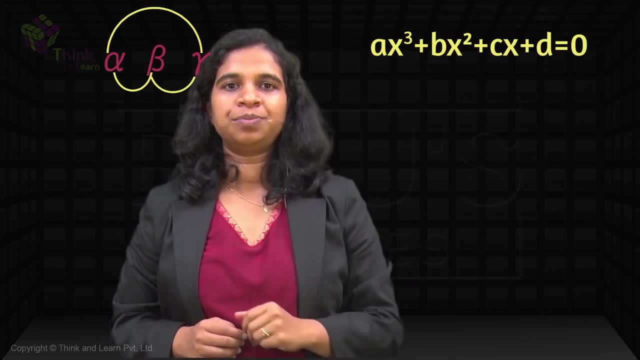 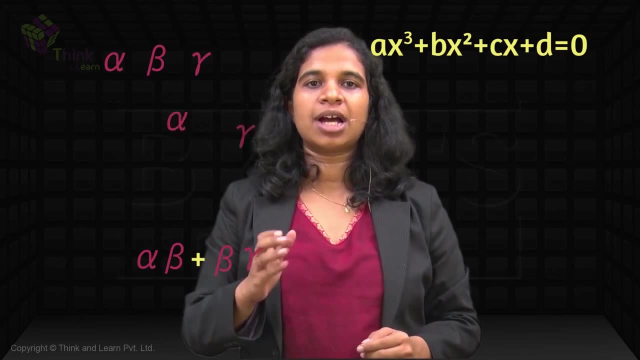 can have alpha and beta, beta and gamma. alpha and gamma. Those are the three possibilities, So add them up. Sum of the roots taken two at a time. So alpha, beta plus beta, gamma plus gamma, alpha. Now sum of the roots taken three at a time. There are only three roots, So 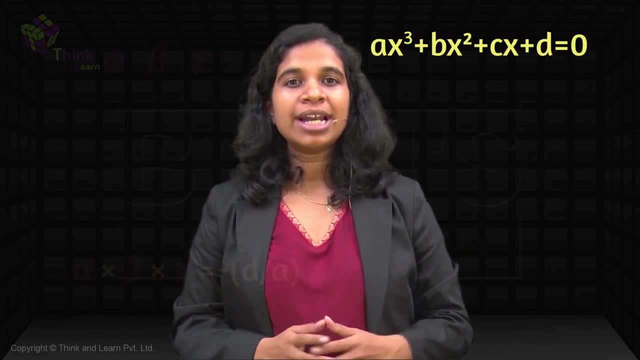 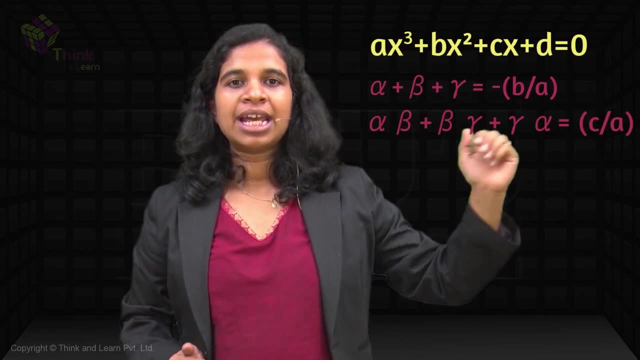 alpha beta gamma. It is the only possibility. So that is what you get. Alpha plus beta plus gamma is minus b by a. Alpha beta plus beta gamma plus gamma alpha is equal to c by a And alpha beta gamma is equal to minus d by a. That's how you get the. 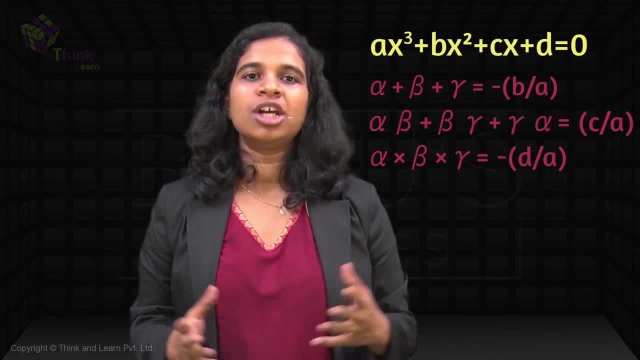 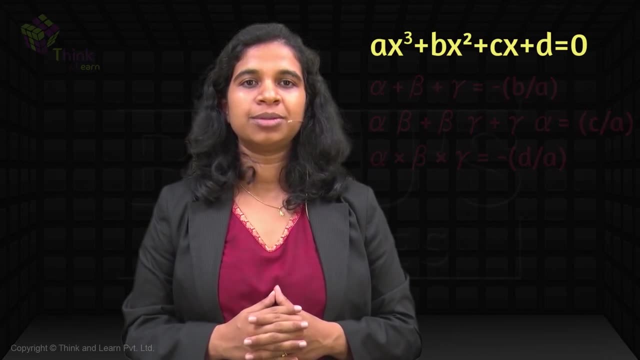 three equations. So again you have three roots and three equations. So very easy to find out the values of all the three. You can very easily find out the values of all the three roots. Same way you can keep extending it Instead of this equation if I make it a fourth power. 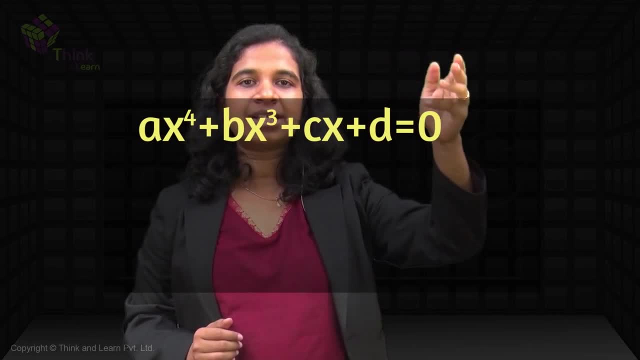 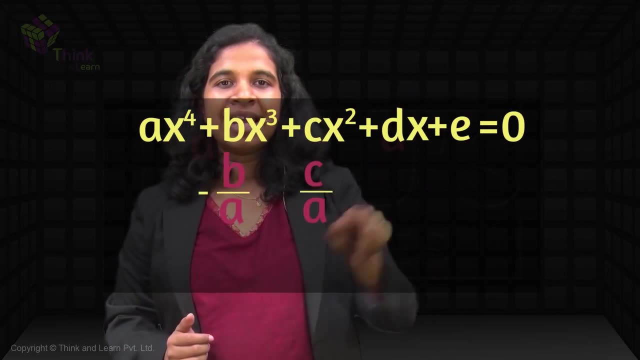 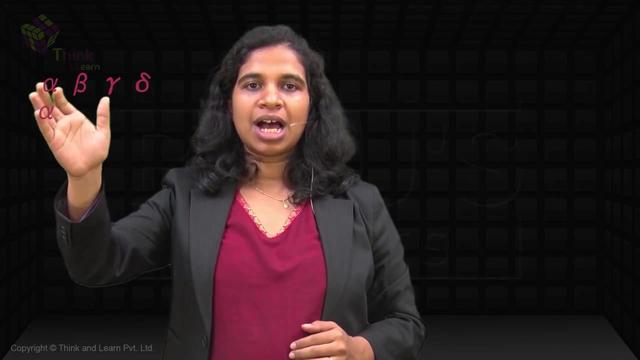 equation right. So we have a? x raised to four, plus b x cubed, Plus c, x squared, plus d x plus e. What do you do? Same thing, Minus b by a plus c, by a, minus d, by a, plus e, by a One at a time. Now you have alpha, beta, gamma, delta, One at a time will be alpha. 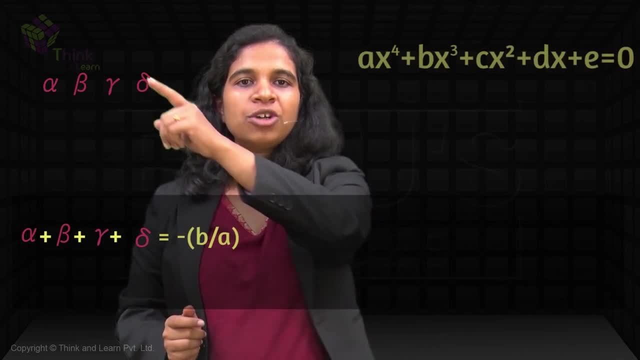 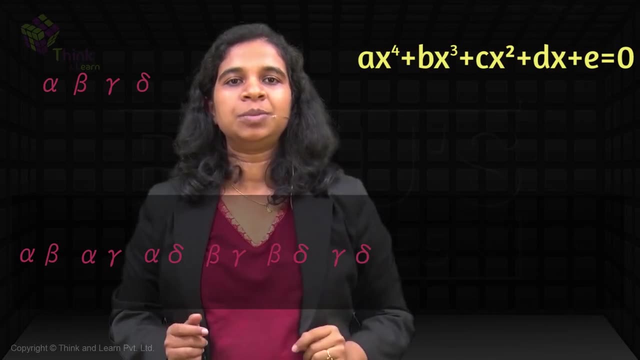 plus beta, plus gamma, plus delta, Two at a time. What all groups can you form? Alpha, beta, alpha, gamma, alpha delta, beta, gamma, beta, delta and finally gamma. Add all those groups up, You will get c by a. 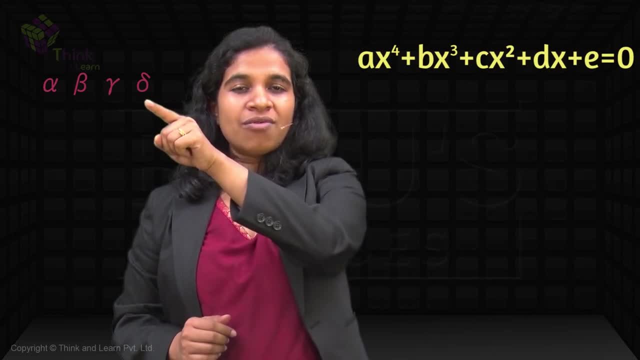 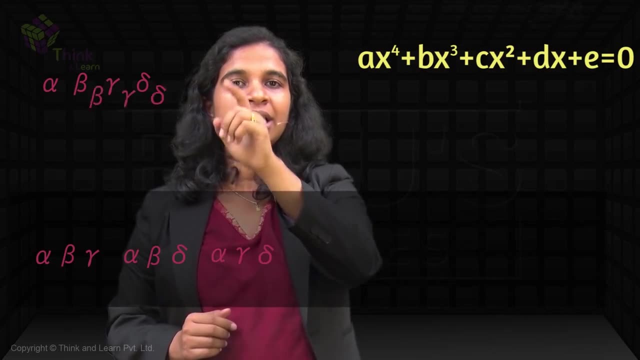 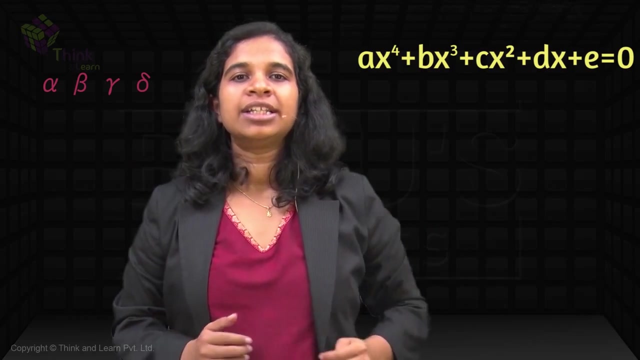 Taken three at a time. How will you take them three at a time? You can have alpha beta gamma, or you can have alpha beta delta, correct, Or you can have beta gamma delta. Those are the only possibilities. Add them up. You will get minus d by Finally taken four at a time there. 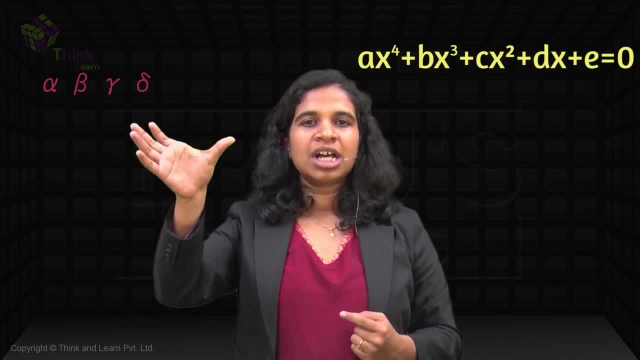 are only four roots, So, taken four at a time, you will have only one term. Alpha beta gamma delta is equal to e by a. Alpha beta gamma delta is equal to e by a. Now you can keep. 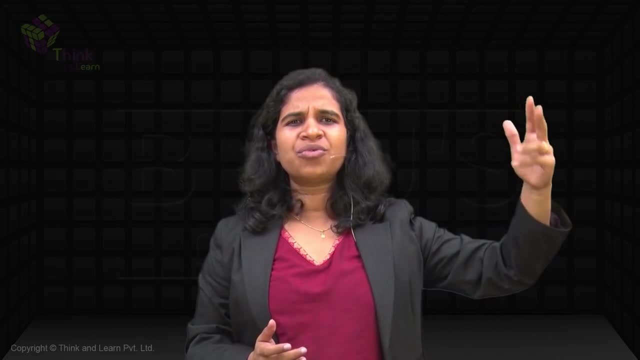 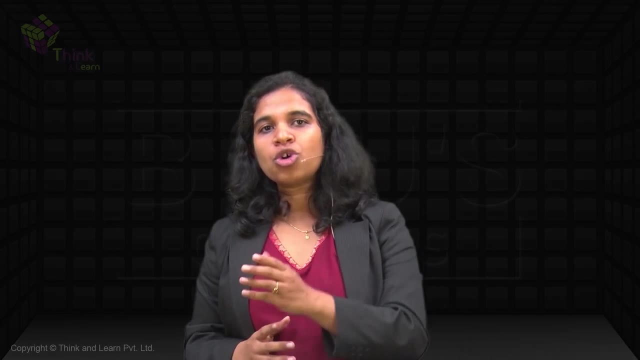 extending this, You get the logic right. Instead of four roots, you will have alpha, beta, gamma. you can have fifth order, sixth order, seventh order, and so on. It does not change. The exact same logic applies. So that's how, if you know the coefficients of an equation, you can very 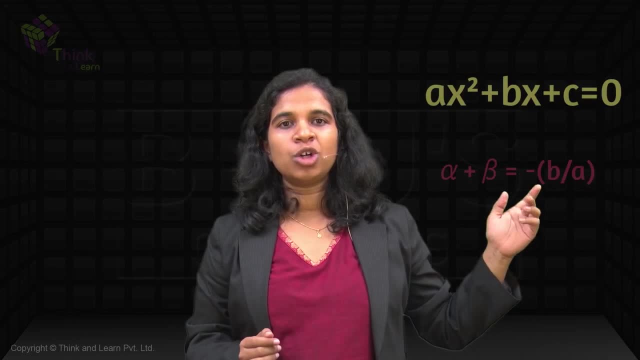 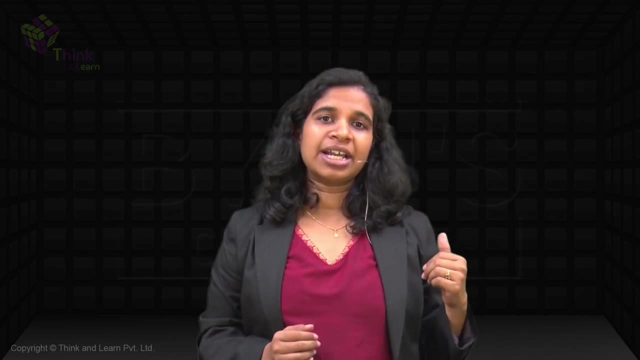 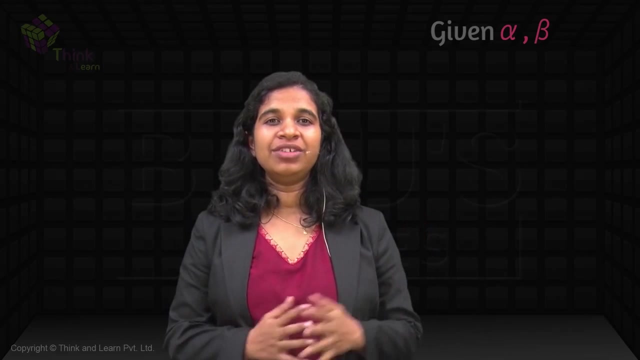 easily find the roots by using alpha plus beta equal to minus b by a. alpha beta equal to c by a. Now can we do the reverse? What if alpha and beta are given to us and we need to figure out a, b and c? Let's see if that is possible. So now we know alpha and beta and we need to figure out. 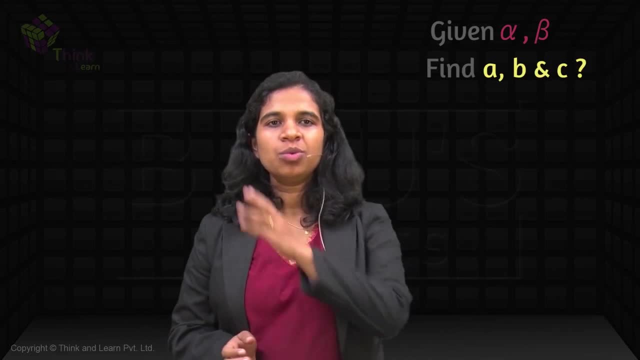 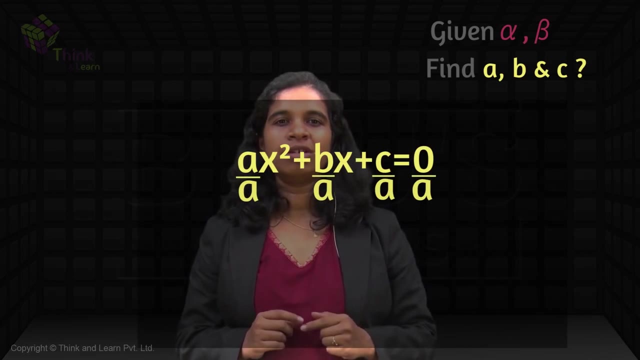 a, b and c. Let's start with our basic quadratic equation. We have a, x squared plus b, x plus c equal to zero. Let's divide both sides by a. As soon as you do that, you will realize why. So we divide both. 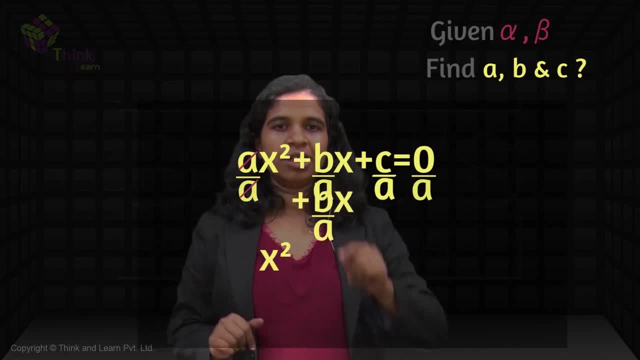 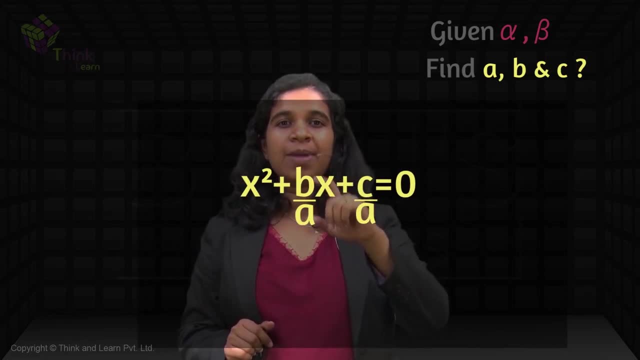 sides by a. What happens here? a and a gets cancelled, So you are left with x. Here you get plus b by a into x, and here you get plus c by a. Now minus b by a is nothing but sum of the roots. 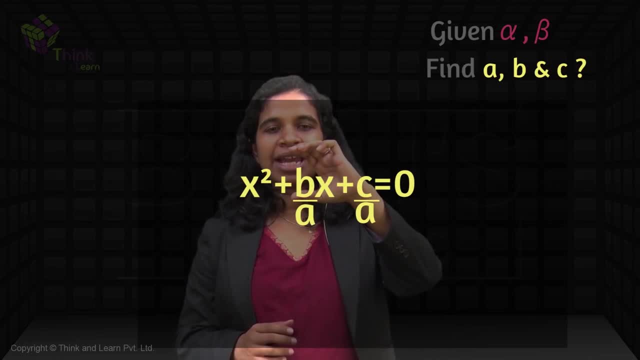 is nothing but alpha plus beta. So in place of this b by a, I can write: this is nothing but minus alpha plus beta. So I can write: this is nothing but alpha plus beta. So in place of this c by a, I can write it as alpha into beta. So in this place I am going to write minus alpha plus beta. 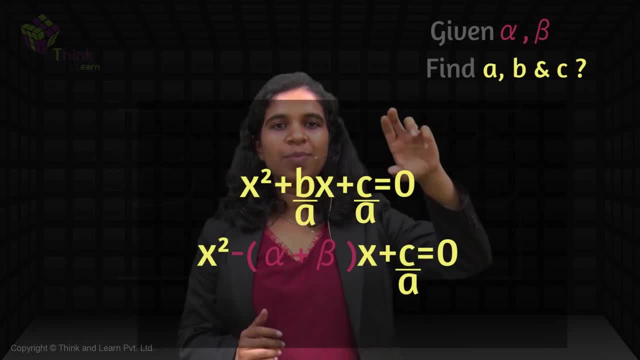 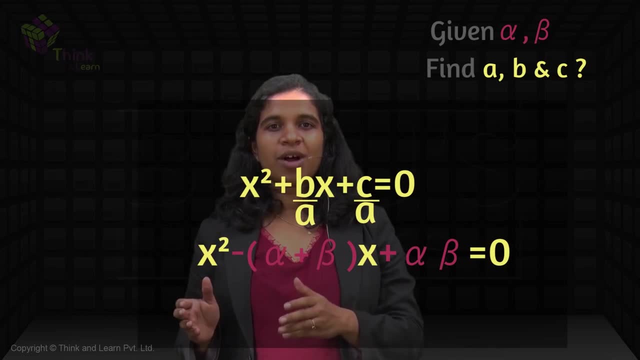 And c by a is nothing but alpha into beta. So in place of this c by a, I am going to write alpha into beta. So what has our equation become? x squared minus alpha plus beta into x plus alpha beta equal to zero. Great, We got our equation from the roots. We knew the roots and we got our. 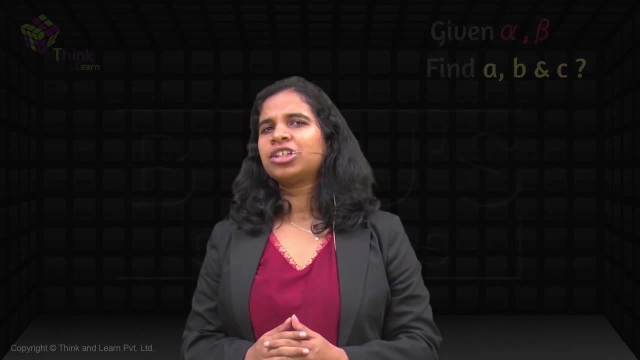 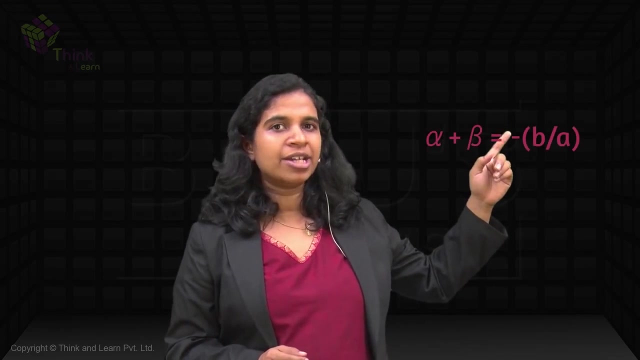 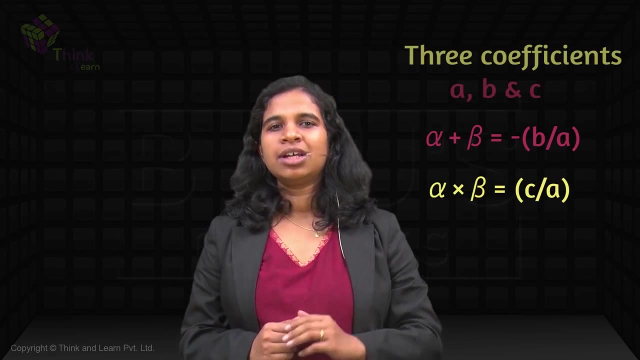 equation Superb. It shouldn't have actually been possible, right? Why am I saying that? How many equations do we have? have just two equations: alpha plus beta equal to minus b by a and alpha beta equal to c by a in the equation that we had. how many coefficients do we have? we have three coefficients: a, b and c. 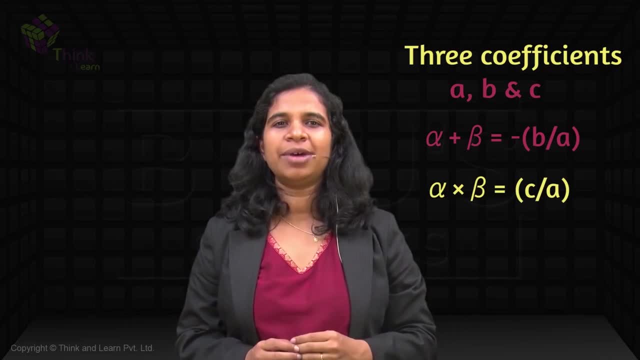 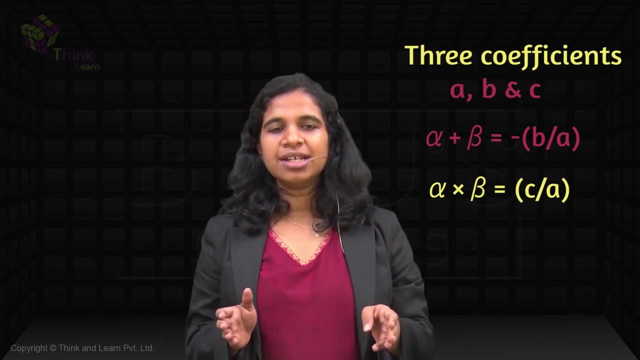 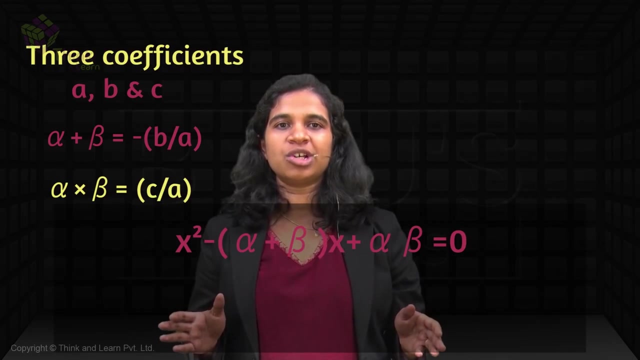 so two equations cannot give you the answer for three variables, right? that's just not possible. so we cannot actually find a, b and c implicitly. what we've done here is we've actually assumed a equal to one. we've assumed a equal to one in writing this equation. that's how we got this. 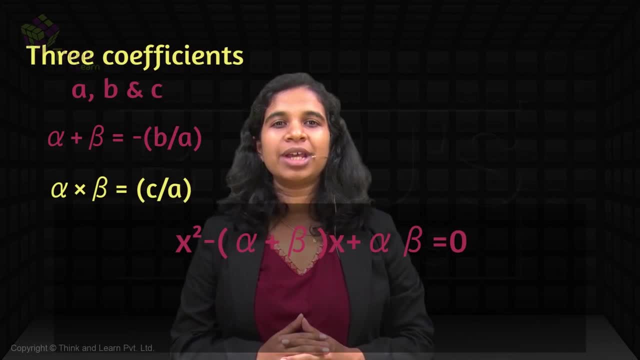 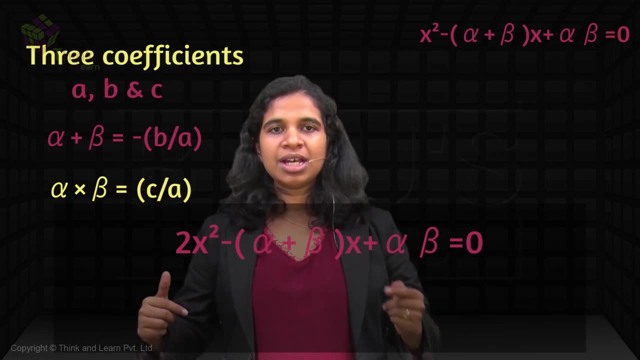 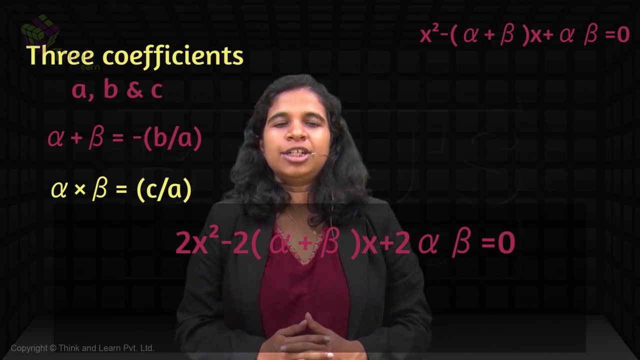 equation right, it's a x squared. now we have only x squared, so we've assumed a equal to one. simple way to think about it is: multiply both sides of this equation by two. what do you get? 2x squared minus 2 times alpha plus beta into x plus 2 alpha beta equal to 0. this is a new. 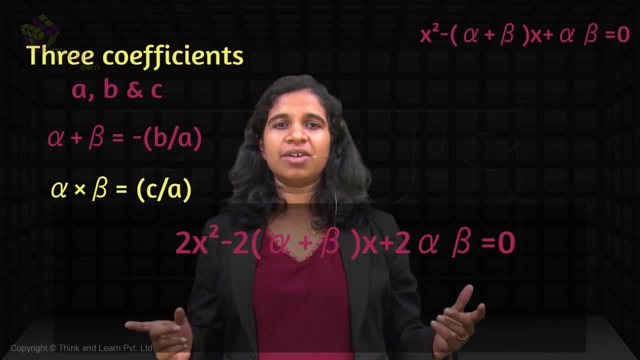 equation. right, it's not the same equation because values of a, b and c are different, so it is actually a new equation. but it still satisfies the fact that alpha plus beta equal to minus b by, because if you divide this equation by two, you get a 2x squared minus 2 times alpha plus beta equal to minus b by. 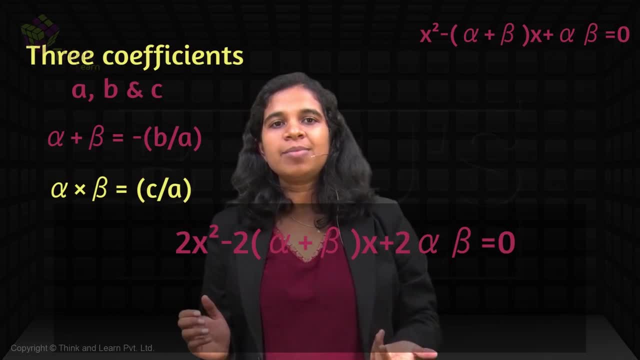 these two, 2 and 2, get cancelled, you get alpha plus beta, And alpha beta will be c by a, because if you divide this and this again, the 2s will get cancelled and you will be left with alpha and 2. 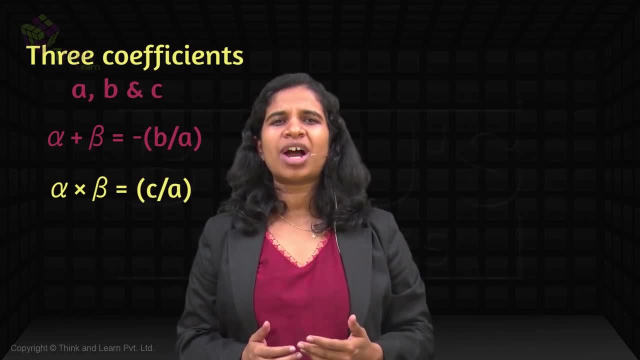 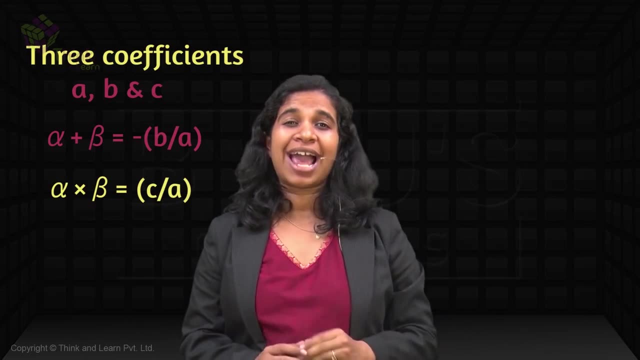 beta. Similarly, I can multiply both sides by 3,, 4,, 5, and so on. I can keep going right. So what will I end up with? I'll not end up with one single equation, but actually a family of equations. 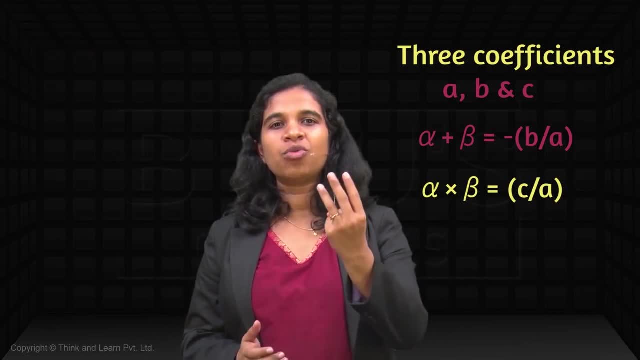 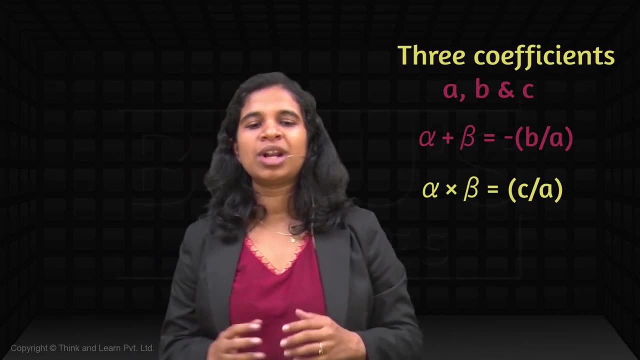 The reason is simple. We have only two equations and we are expected to find three coefficients. It's just not possible. You will always get infinite solutions. It's much easier to visualize this on a graph. Let's take an example. Let's say alpha equal to minus 3 and beta equal to 1.. 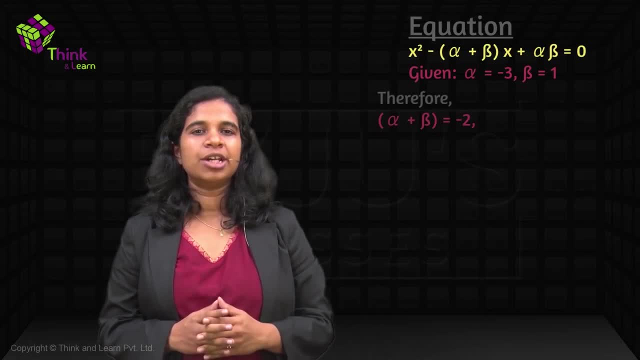 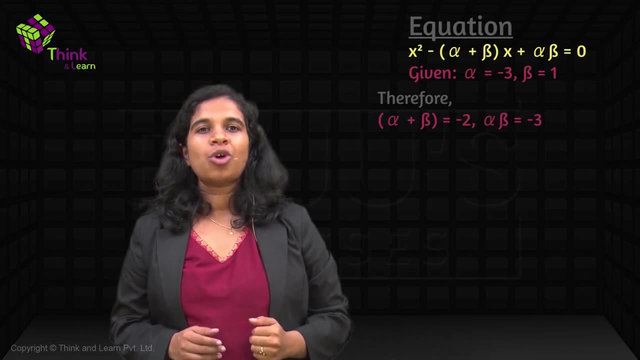 What is the value of alpha plus beta? You'll get minus 3 plus 1, which is minus 2.. So alpha plus beta is going to be minus 2.. Alpha into beta will be minus 3 into 1, which is minus 3.. So alpha plus. 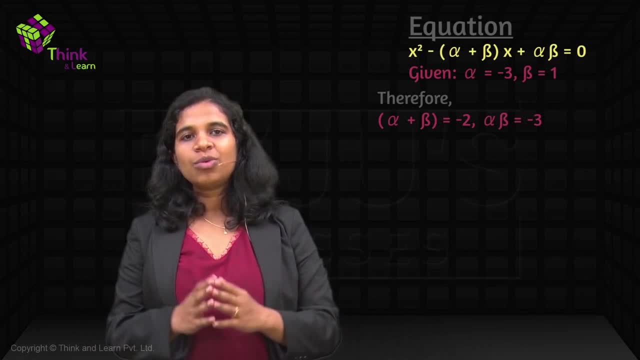 beta is minus 2, alpha beta is minus 3.. What was our equation? We said equation is x squared minus alpha plus beta into x squared. So alpha plus beta is minus 2, alpha beta is minus 3.. So alpha plus. 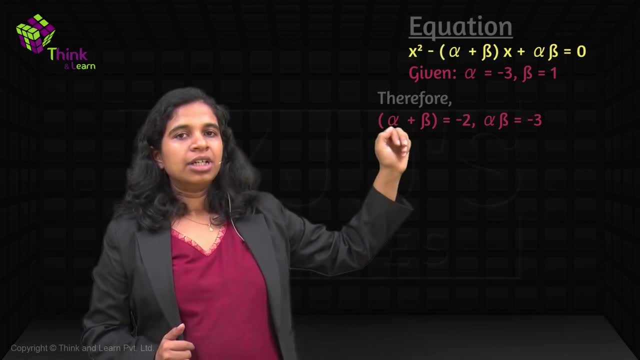 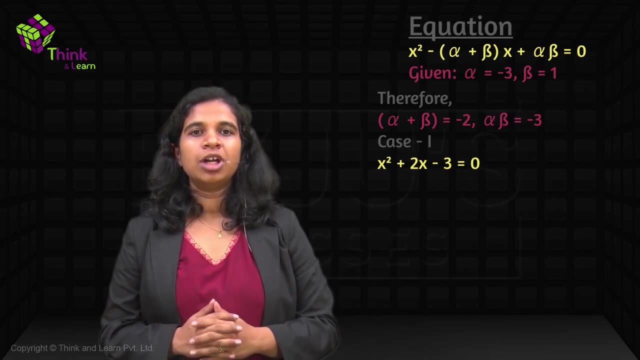 2x plus alpha beta, equal to 0.. So x squared plus 2x minus 3.. That's what our equation will be right, Because minus of minus 2 becomes plus 2.. So x squared plus 2x minus 3.. Let's draw it on a. 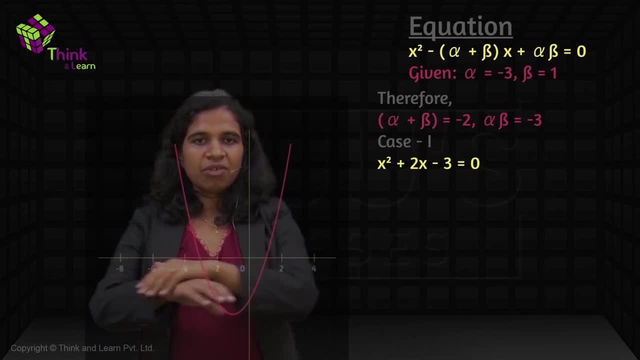 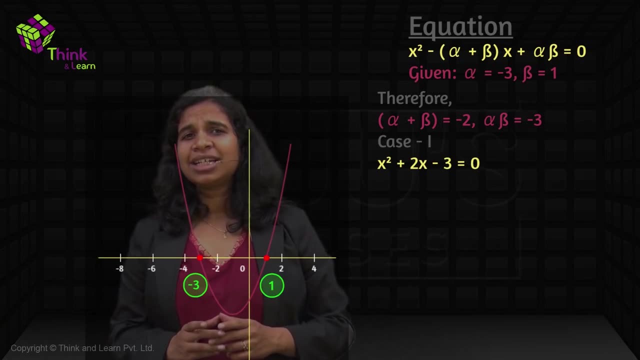 graph. So I'll get x squared plus 2x minus 3.. If I draw my x-axis here, I'll get alpha and beta here. So I have alpha and beta. Now. what we are essentially saying is, instead of having this, 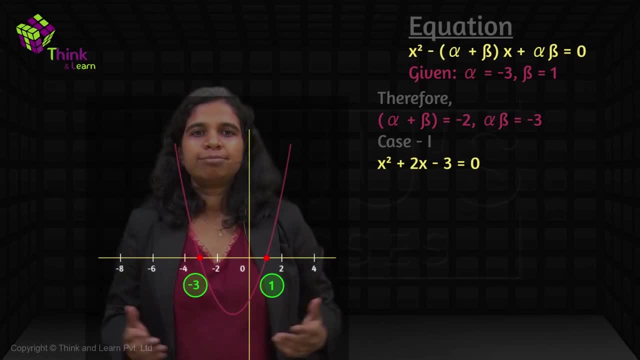 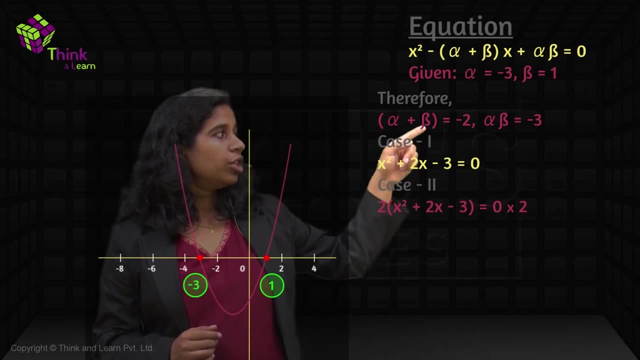 the same equation. can I multiply both sides by 2? Possible, right? Nothing is changing. I'm allowed to do the same operation on both sides. So if I multiply both sides by 2, I'm going to end up with 2x squared plus 4x minus 6.. 2x squared plus 4x minus 6.. 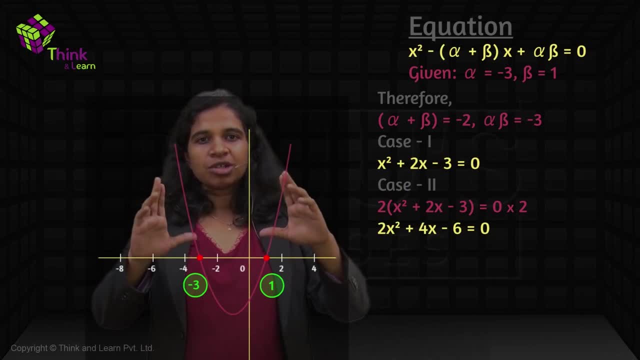 Now 2x squared. So what is going to happen to this equation? It's going to become steeper, right? We know that the coefficient of x, that is, a, steepens our curve. As a increases, the curve becomes steeper, So it actually closes. So this graph is going to look something like this: 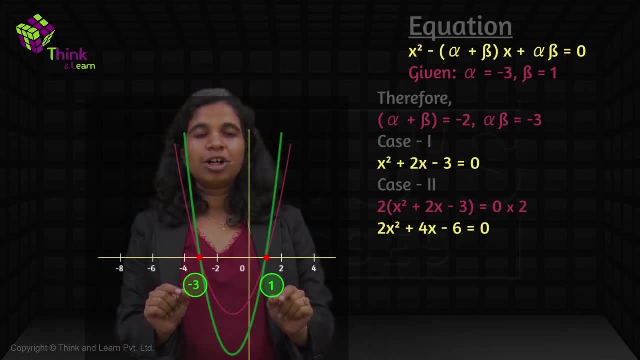 Notice it cuts the x-axis at the same two points because the values of alpha and beta are the same. So this is your equation: 2x squared plus 4x minus 6.. So notice, both of these are different equations. right? We have different graphs. They are not the same equation, They are different. 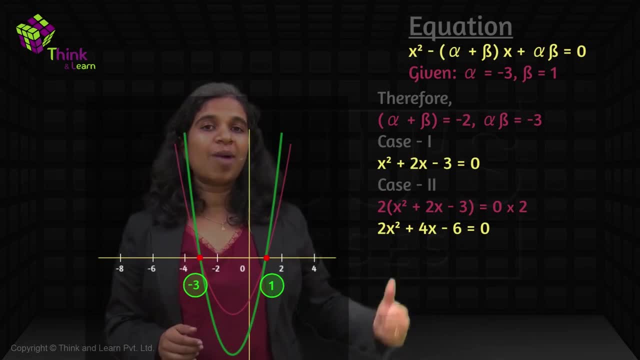 equations, but they have the same root. Let me take a third one. Instead of multiplying by 2,, let's say I divide by 2.. So I get half x squared plus x minus 3 by 2, equal to 0.. Try drawing this. 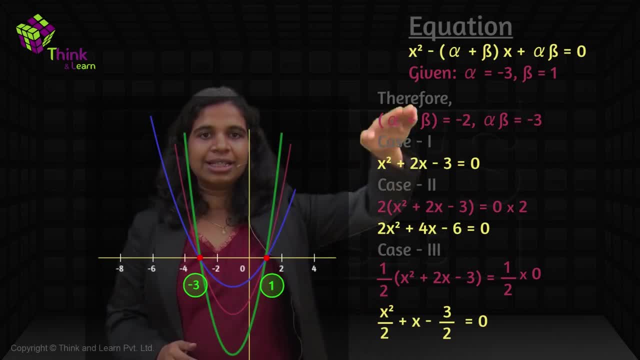 What will happen? The original graph will open up, right, So you'll get an equation like this Again, passing through the same two points on the x-axis. So alpha and beta are the same, but it's a different equation. Clearly it's a different curve, right, The graph is different. 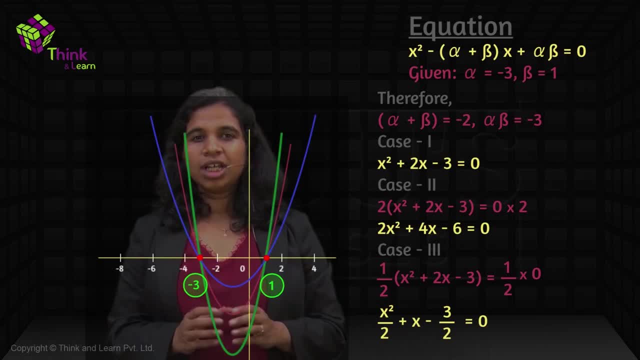 So all of these three are actually different equations. The curves are different, They're different polynomials but have the same roots. They're different polynomials but they have the same roots. Why? Because we have only two equations, So we can keep multiplying it by. 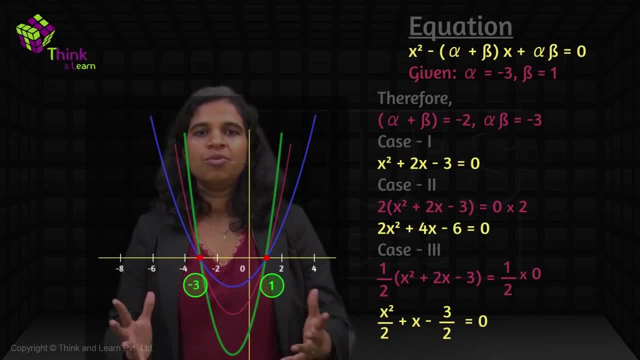 two, So we can keep getting more and more equations. You can have an infinite number of equations here. We just plotted three sample ones. All of these are equations where both roots are common. Now, mathematically you'll get some questions based on common roots. There's nothing. 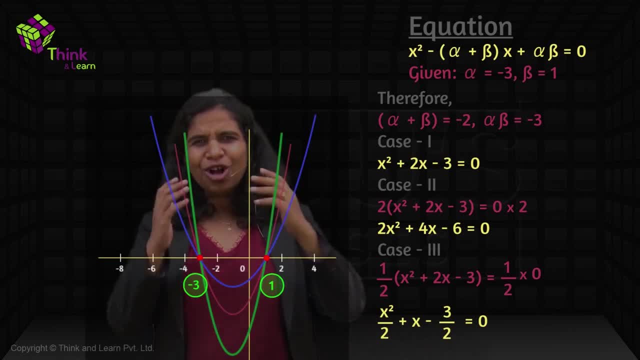 different. It's not a topic to be learned separately. common roots, It's all common sense at the end of the day, You don't have to learn subtopics like that. Common roots is a different topic. It's not a different topic. Once you know this concept, you can easily find These. 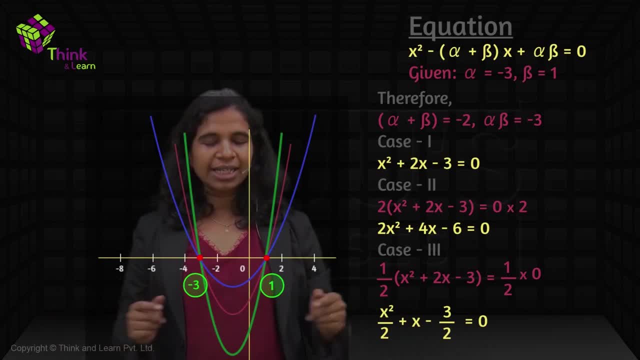 are nothing but equations which have both roots common, correct? Because these are common roots. they are cutting the x-axis at the same two points. so they have both roots common. now, what is? what do you see? is the similarity between these equations. we've written these one below the other. 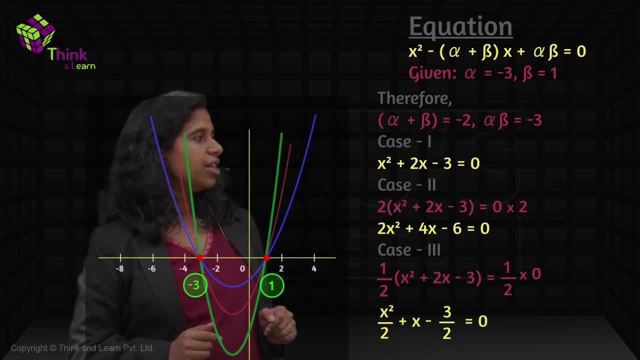 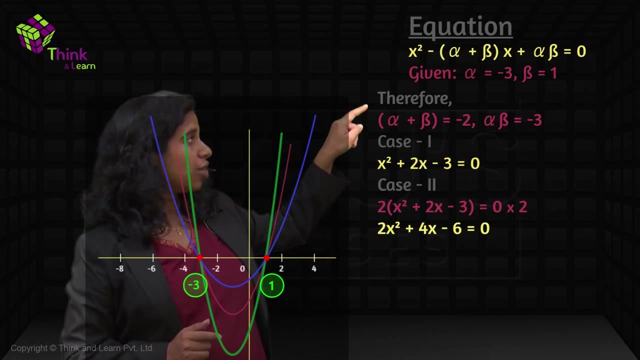 right, we've written this one below the other. now what do you see here? look at the coefficient of x. look at the coefficient of x. take just the first two equations. here you have x squared plus 2x minus 3. here you have 2x squared plus 4x minus 6. coefficient of x squared is 1 and 2 coefficient. 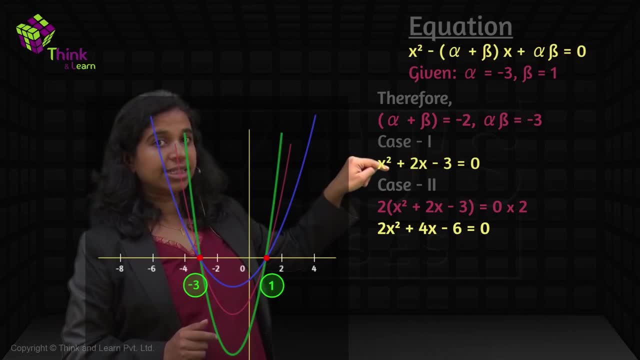 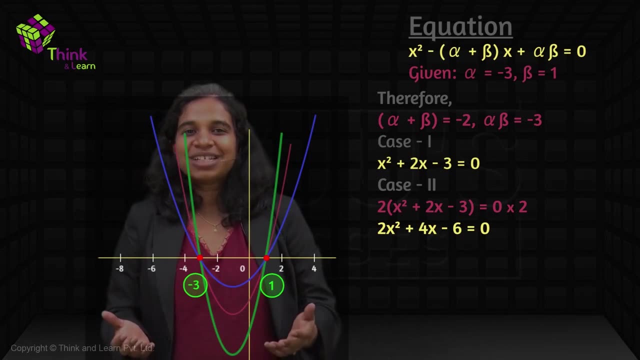 of x is 2 and 4 and the constant is minus 3 and minus 6. do you notice some similarity? the ratio is same. right, it will obviously be the same. that's how we got the second equation in the first place. we got the second equation by multiplying by the second the first one by 2. 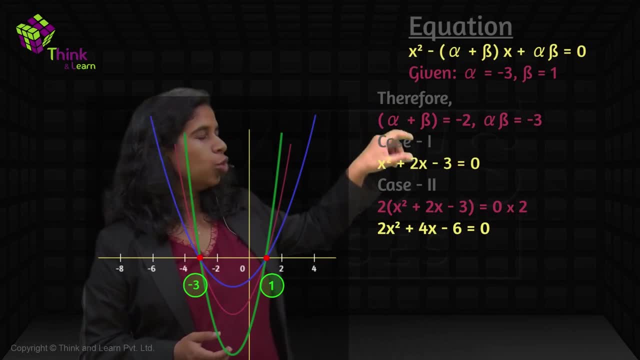 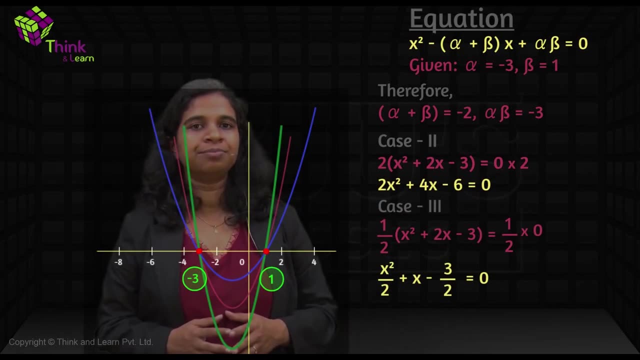 so the ratio is 1 by 2 right, 1 by 2, 2 by 4 is nothing but 1 by 2. minus 3 by minus 6 is nothing but 1 by 2. similarly, compare the second and the third one right. what is the coefficient of x? 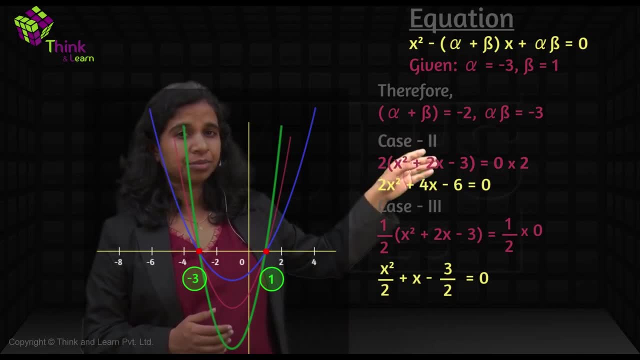 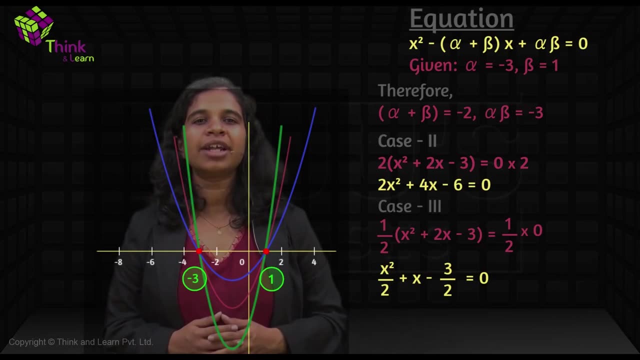 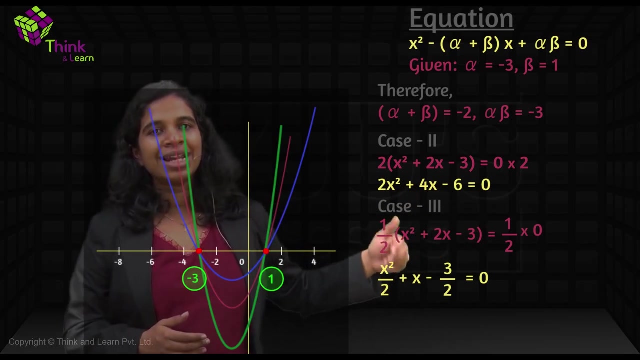 squared here: 2 and 1 by 2, here it is 4 and 1, here it is minus 6 and minus 3 by 2. again, find the ratio. it's nothing but 4. everywhere the ratio is 4 right. 2 by 1 by 2 is 4, 4 by 1 is 4. minus 6 by minus 3 by 2. 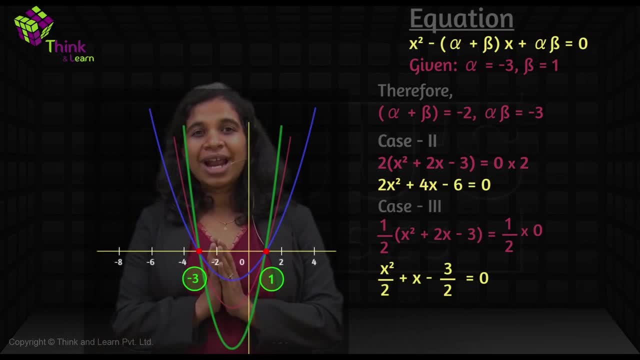 is 4. so what do you see here? if we had to write an algebraic, this is the graphical representation, right, they are all cutting the x-axis at the same two points. if we were to write this mathematically, if i call the coefficients of x squared x and the constant as a1, b1, c1 for the first equation, 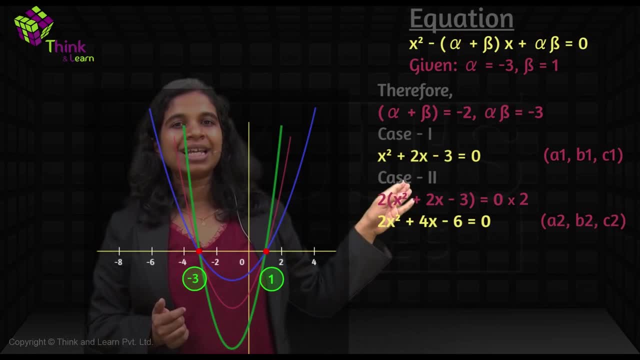 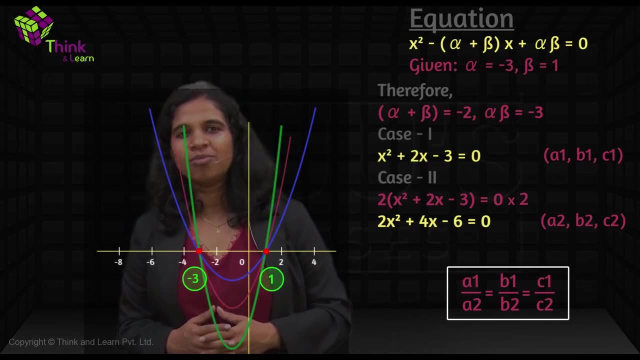 and a2, b2, c2. for the second equation. what we are basically saying is that a1 upon a2 will be equal to b1 upon b2, will be equal to c1 upon c2, which is obvious, right? that's how we get the second. 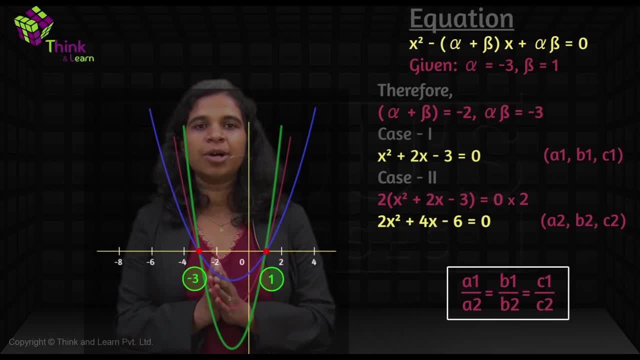 equation. so whenever you have both roots common in a particular equation, the ratio of the three coefficients will always be constant. so your a1 by a2 will be equal to b1 by b2 will be equal to c1 by c2, and this is how they look. different shapes, but cutting the x-axis at the same point. 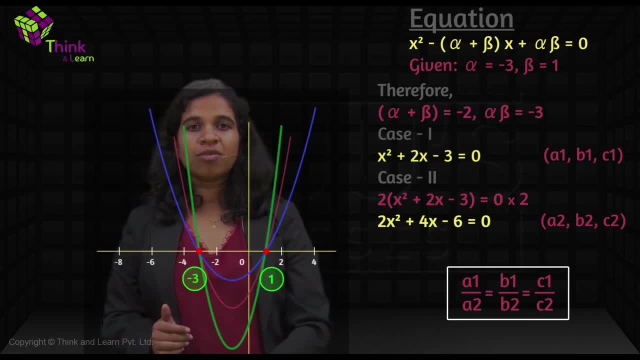 the horizontal position. the horizontal position of their vertex will also be the same. see, if i draw this straight line, all the vertices are falling on this line. can you tell me why? where does the vertex lie? minus b by 2a and minus b by a is the same for all of them, right? 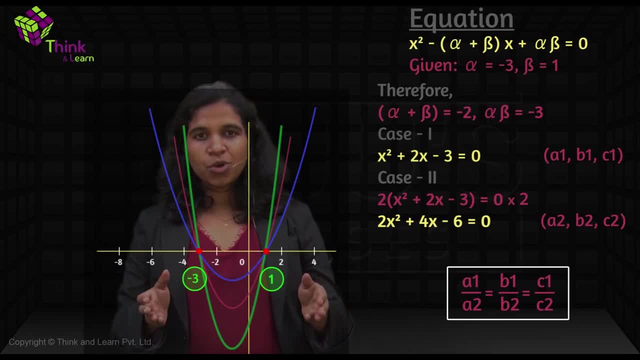 because minus b by a is nothing but the sum of the roots. so the sum of the roots is the same, so minus b by a is same, hence minus b by 2a. it also has to be the same, so logically, their vertex will lie on the same vertical line, the. 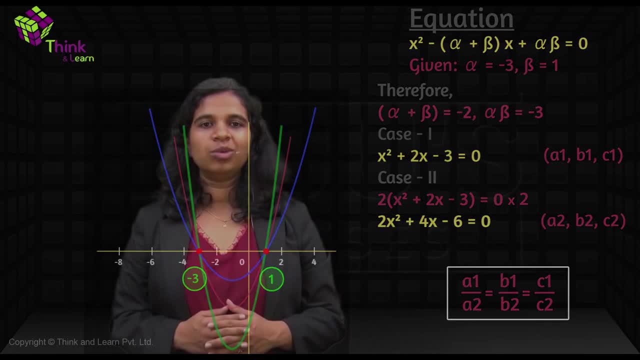 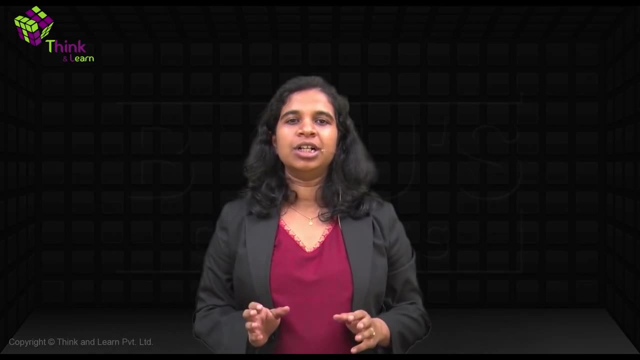 x coordinate will be the same, the y coordinate will vary, the y coordinate will vary. so that is, equations where both roots are common. if only one root is common, then it's very, very simple. if you get an equation where only one root is common, it's very simple to solve it. so two roots: 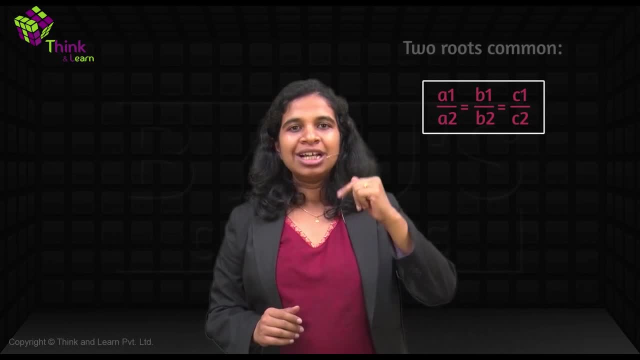 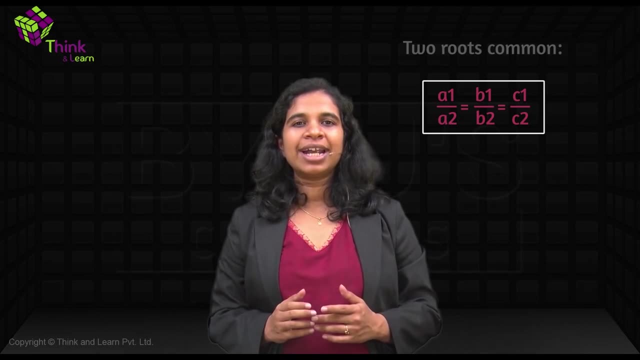 common. you know, this is the relationship. if one root is common, just equate the coefficient of x squared. just equate the coefficient of x squared and then subtract the two equations, so x squared will get cancelled and you will just be left with x. so you will easily be able to find what. 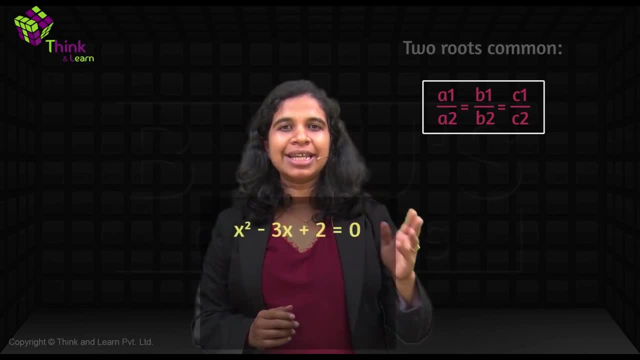 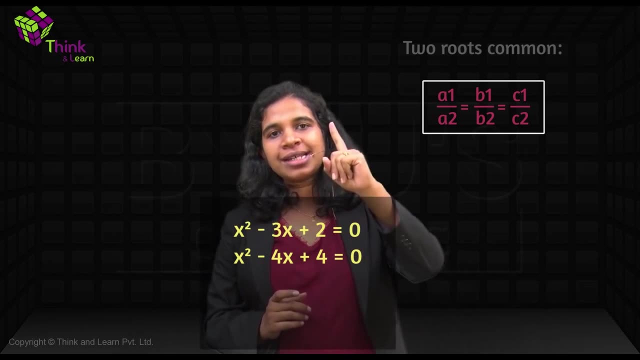 the value of the common root is. so suppose i have x squared minus 3x plus 2 equal to 0 and i have x squared minus 4x plus 4 equal to 0. these are the two equations. first step, i told you, is equate the coefficient of x squared. luckily for us here x square has the same coefficient. 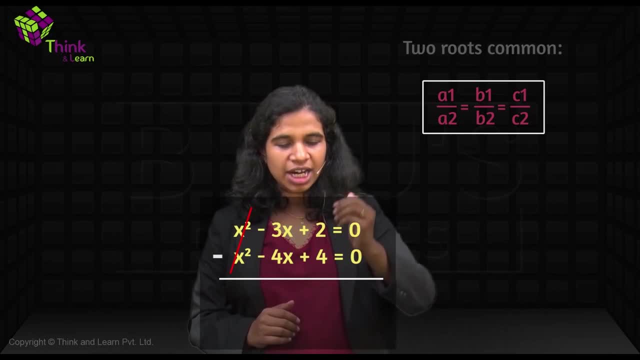 so i'll subtract x squared and x squared get cancelled. right you are. I get minus 3x plus 4x. minus and minus will become plus right, so it will be x here. I get plus 2 minus 4, so it becomes minus 2. so what you're left with is x minus 2 equal to 0, which means x is equal to. 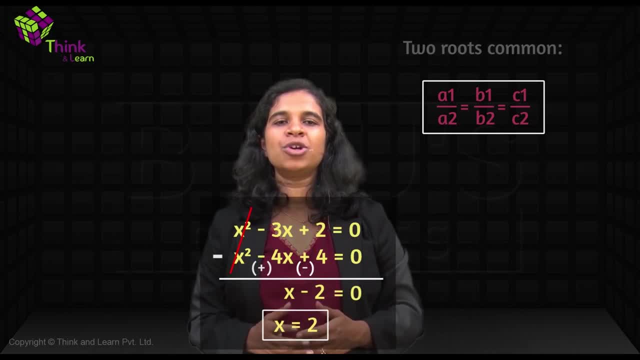 2. so that's the common root for these two equations. the common root is: x is equal to 2. first equation has roots 2 comma 1. second equation has roots 2 comma 2. second equation is nothing but x minus 2, the whole square right. you can see that. so that's how you'll do: both roots common. 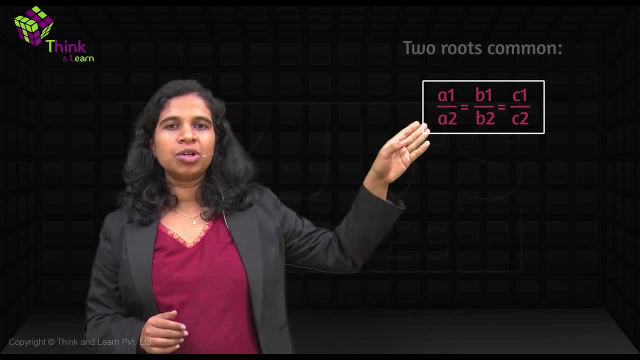 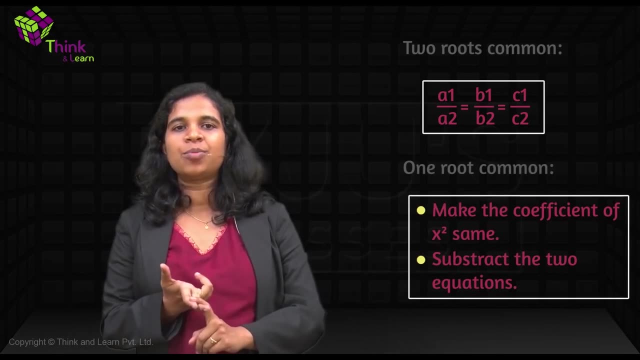 both roots common. we have a1 by a2, equal to b1 by b2, equal to c1 by c2- only one root common. two simple steps: make the coefficient of x squared the same and then subtract the two equations so your x squared will get cancelled. you'll be left with a linear equation. you can solve it to. 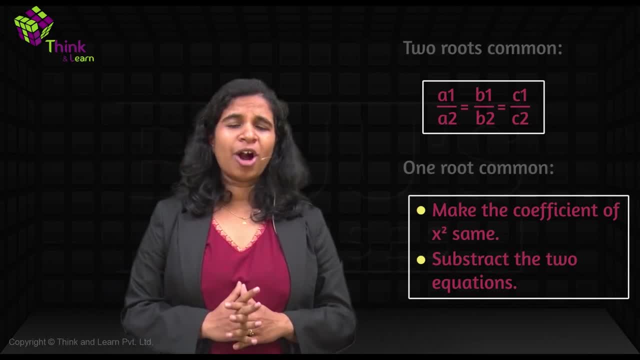 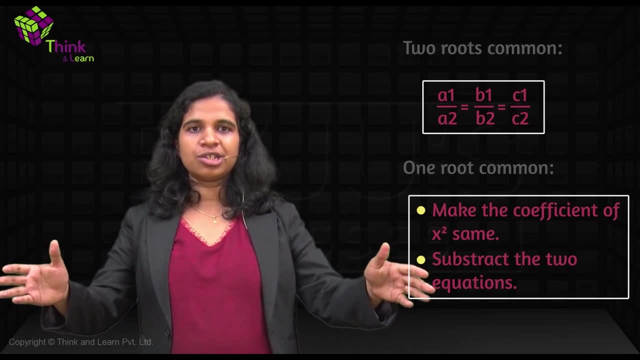 find the one common root. that's how you'll find common roots. what is more important here is to know that when roots are given, you cannot find a unique equation. what you'll get is the family of equations, like we saw earlier, all of them cutting the x-axis. 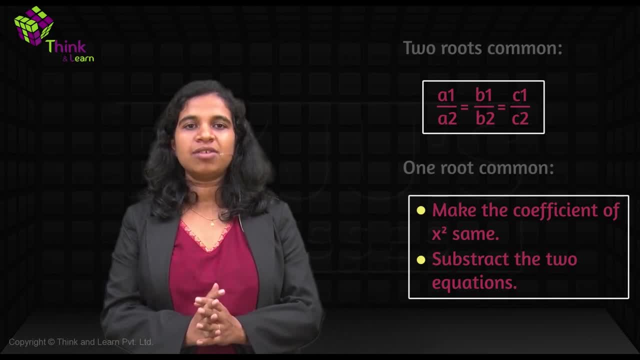 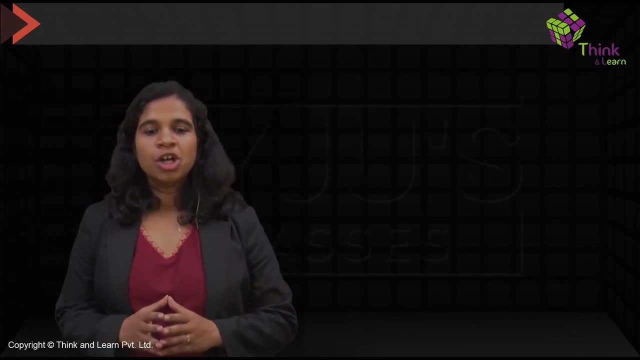 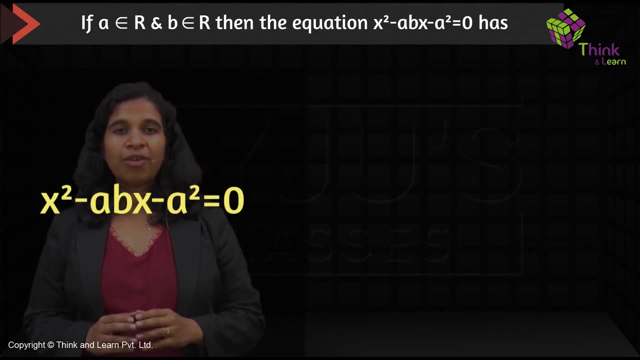 at the same two points because they have the same roots. it's a family of equations where this particular condition is true: a1 by a2, equal to b1 by b2, equal to c1 by c2. so the equation we had was x squared minus ab into x minus a squared equal to 0. you need to find out what the nature. 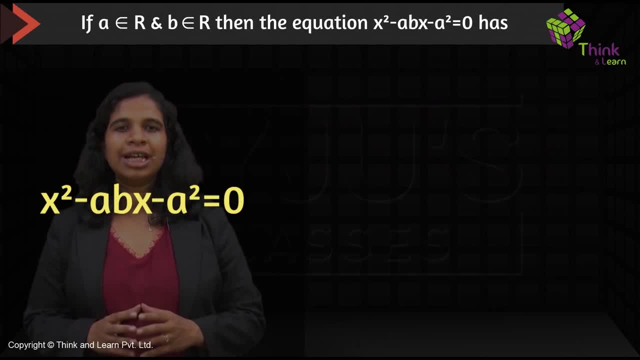 of the two roots are in terms of whether they are positive, negative and so on. see, whenever you have to find positive and negative, it's always useful to take the product rather than the sum. why the product? because you have a common root and you have a common root and you have a common root. 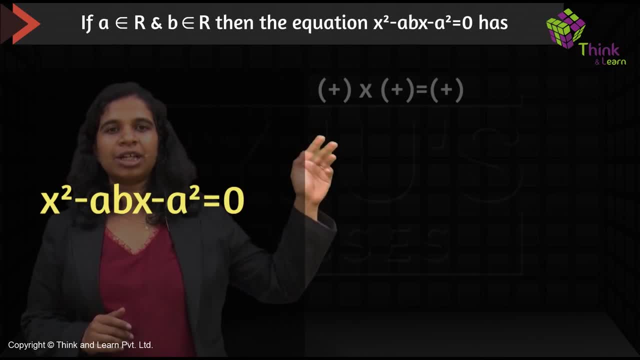 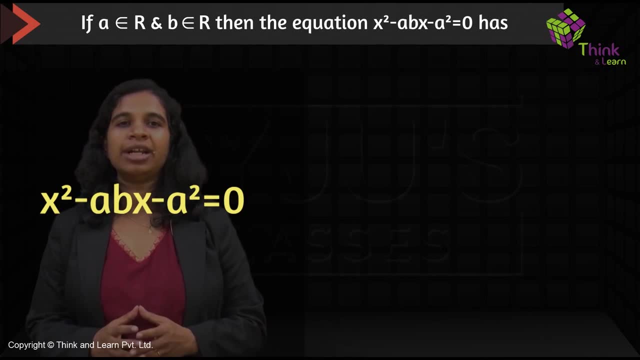 so the answer is: what if i take the property 1 and i derive 1? well then i'm adding the right number to 1, then i'll subtract good and bad. all right now. note Gent oppenheim here: jar highway, because we have a common root. 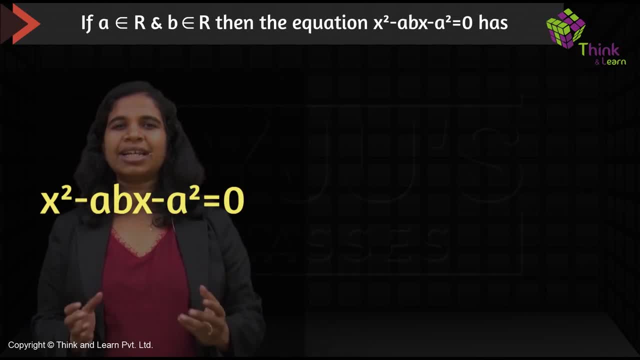 numbers never helps you in trying to find the nature of the two. Only thing that can help is product. Let's see what the product is. That's why we look at product of the roots. So what is product of roots? Alpha into beta is c by a. c here is minus a, squared a is 1.. So alpha into beta. 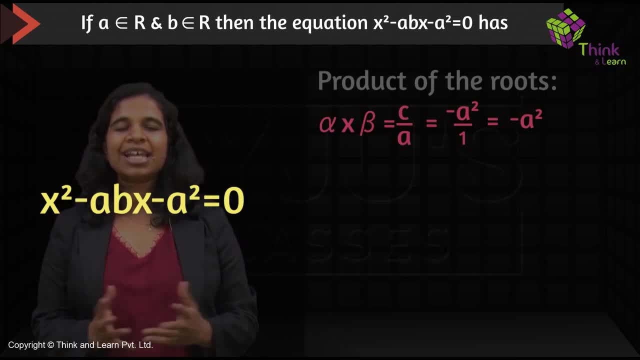 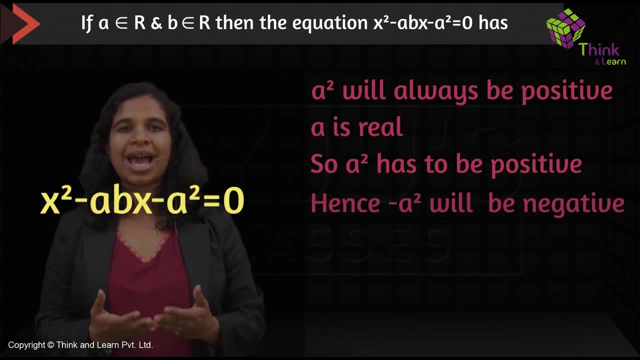 will be minus a squared by 1, which is minus a squared. a squared will always be positive. right a is real, not imaginary, So a squared has to be positive, which means minus a squared has to be negative. So sum of the two roots is negative. Look at the table we just wrote. Where do you get? 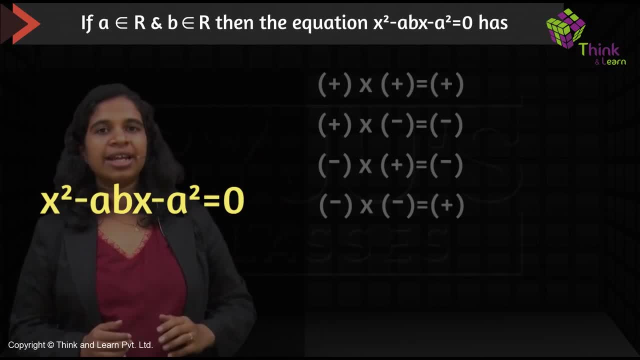 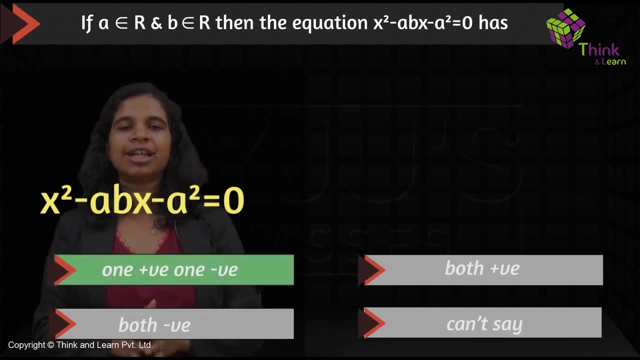 a negative value. When 1 is positive and 1 is negative, right Either plus into minus or minus into plus. So basically, 1 root is positive, 1 root is negative. That's why you get your answer as option a, which is: 1 root is positive, 1 root is negative. So remember this when you're trying. 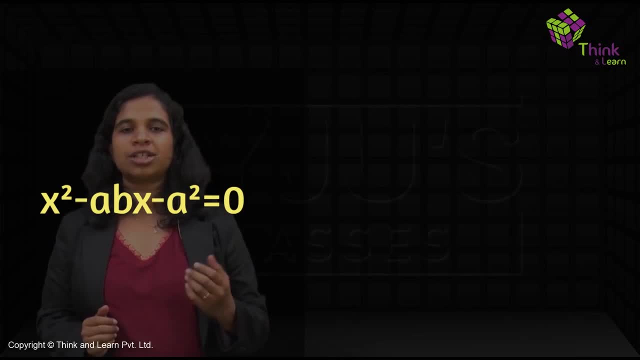 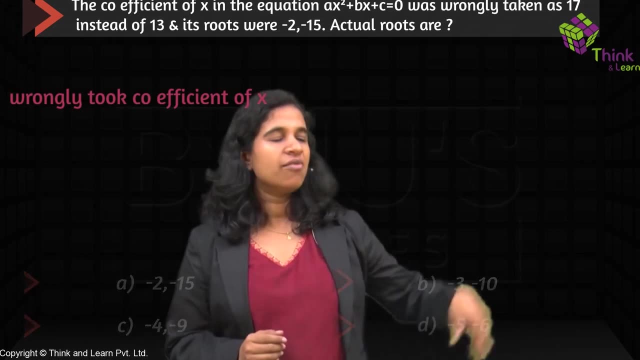 to find the positive or negative nature. always look at product and not sum. There are two cases here. The person basically goofed up the coefficient of x. What is the coefficient of x? If you look at a x squared plus b, x plus c, the coefficient of x is: 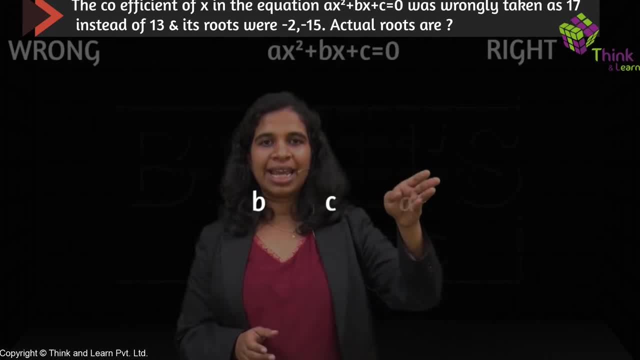 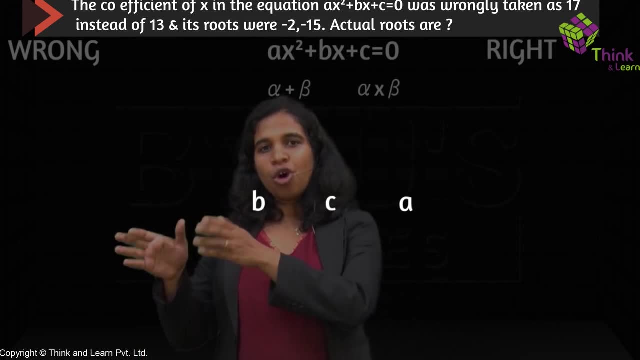 b. So let's take the two cases. So we have b, c and a, which are the three coefficients, and then you have alpha plus beta, alpha into beta. The wrong case and the right case Now in the wrong. 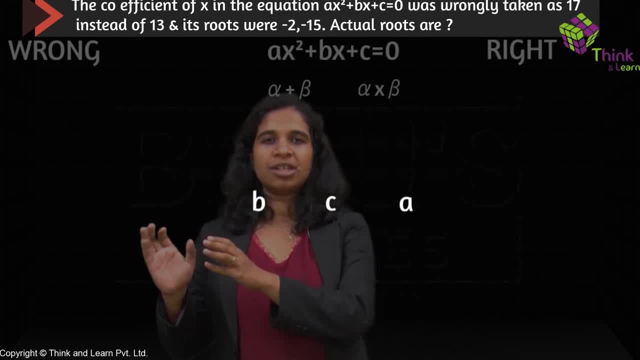 case, what did the person mess up? He messed up the coefficient of x. So he messed up the value of b. He took b as equal to 70, when he was actually supposed to take it as 30. So the right value was. 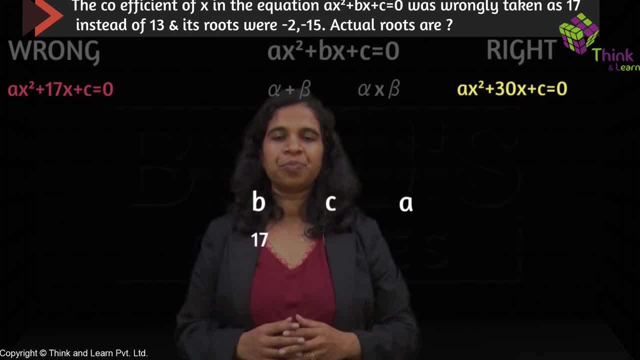 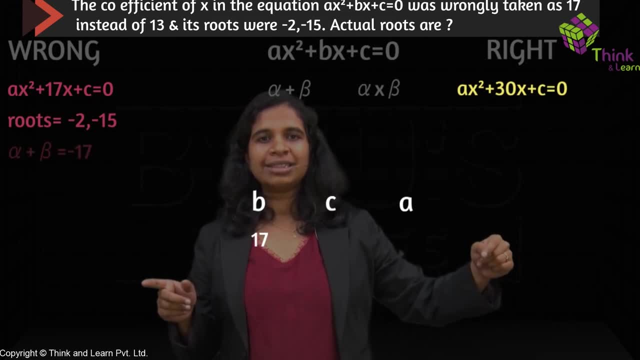 13.. The wrong value was 70.. c and a. he didn't mess. Now what is the roots that he got In the wrong case? his roots were minus 2 and minus 15.. So what is sum of roots Minus 70.. Product of roots: 30.. Sum of roots is: 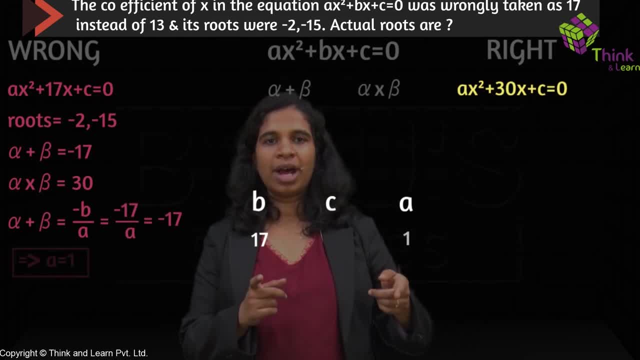 minus b by a, b is 70. What will a be equal to 1.. c by a is product of roots, which is 30. So c will be equal to 30, right 30 upon 1, equal to 30. Now a and c in the case where he got it. 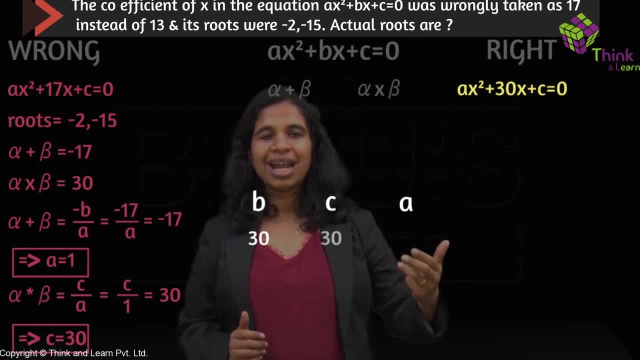 right, he didn't mess up a and c, So he still took c as 30 and he still took a as 1.. So now, what were his values of b, c and a, 13,, 30 and 1.. What will be sum of roots Minus b by a? 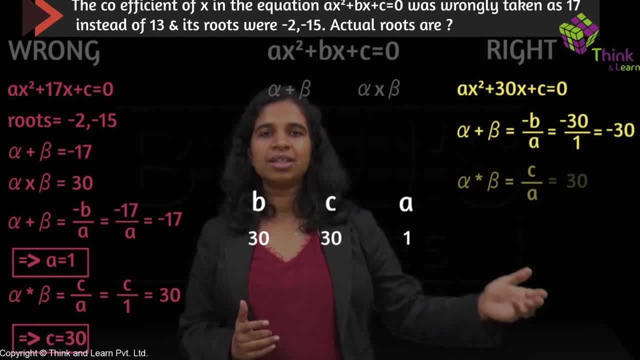 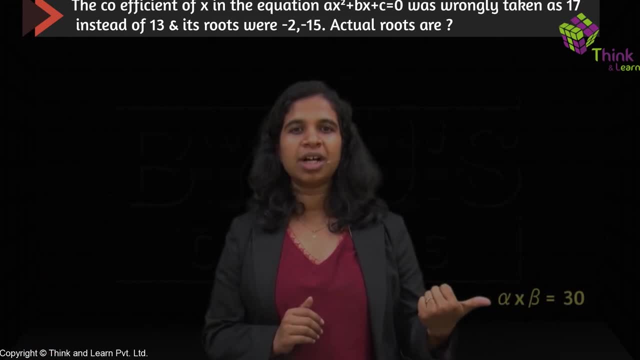 minus of 13 by 1, minus 13.. Product of roots c by a: 30. So now we know that sum of the roots is minus 13,. product is 30.. Now just look at your answer options. So you know product has to be 30.. 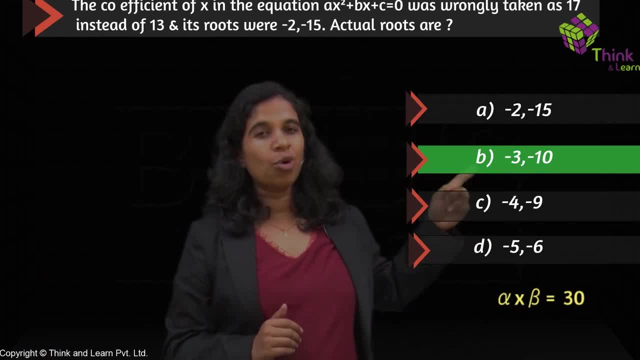 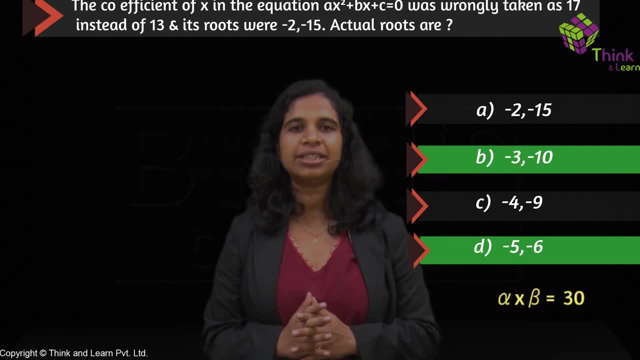 If you check where you're getting the product, 30,. out of the four options, only b and d give you the product as 30. Only b and d give you the product as 30. So you can simply eliminate a and c. The answer has to be one of b or d. Now check which of the two give you a sum of minus 30.. 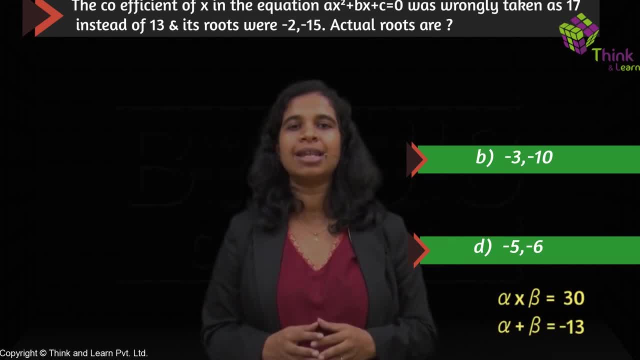 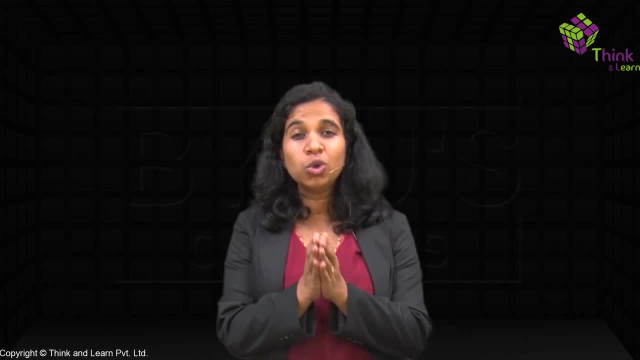 Only b gives you minus 30, right. In case of d, the sum will be minus 11.. So you can eliminate d. You're left with only option b. So always keep looking at the answer options and use the reverse.